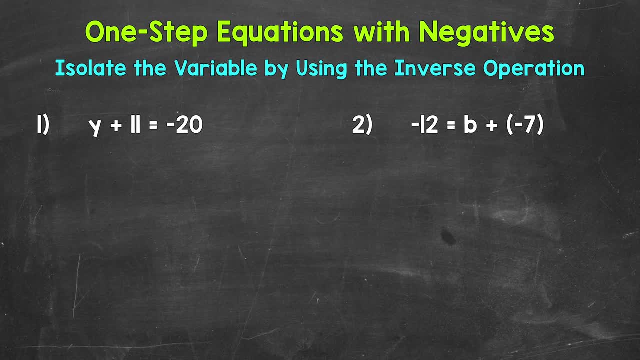 we solve them the same way. we solve one-step equations that have only positives. We want to isolate the variable, which means get it by itself, And we do this by using the inverse operation, which means the opposite operation. Basically, we want to undo whatever is being done to the variable. 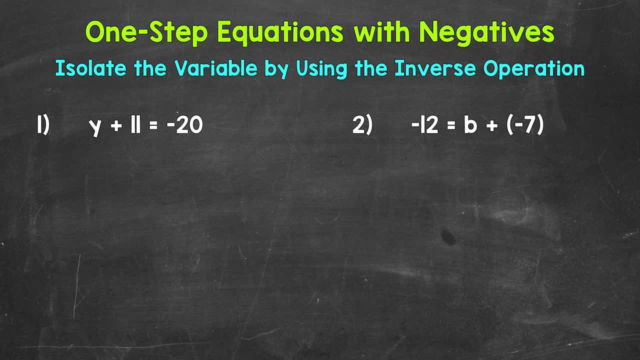 That way, the variable is by itself on one side of the equation. And again, we do this by using the inverse or opposite operation. Just remember: whatever is done to one side of the equation, it must be done to the other in order to keep everything balanced and equal. 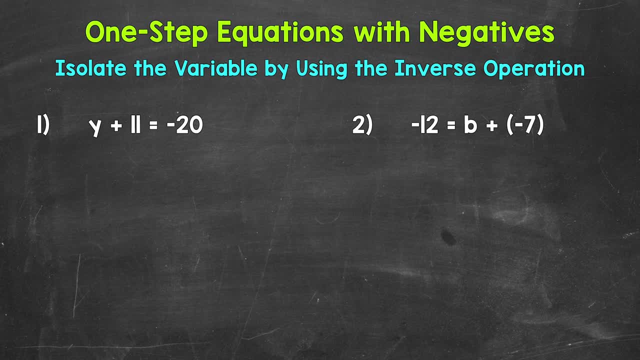 Let's jump into number one, where we have: y plus 11 equals negative 20.. Now we need to isolate that variable of y. We need to figure out what y equals. Since 11 is being added to y, we need to undo that addition by using the inverse operation. 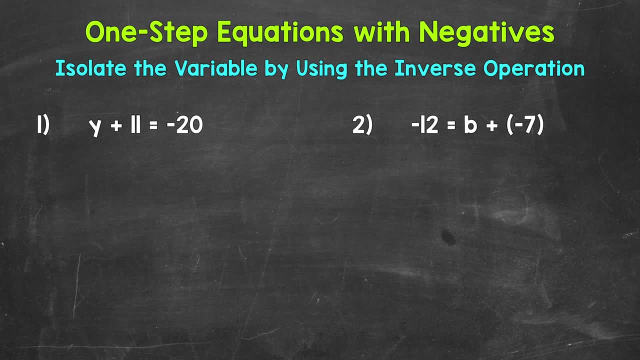 so the opposite operation, The other way around, The opposite of addition is subtraction. So let's subtract 11 from the left side of the equation. Now, whatever we do to one side of the equation, we must do to the other in order to keep it balanced and equal. 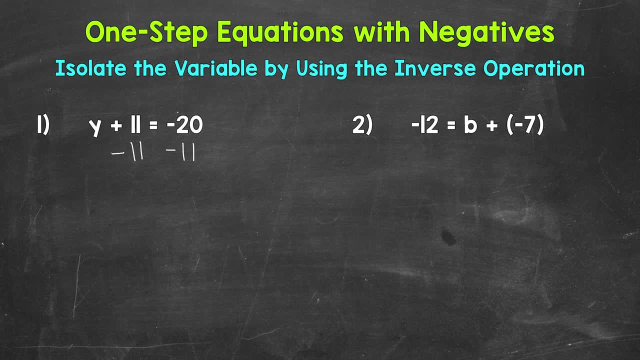 So let's subtract 11 from the right side as well. Now, if we take a look at the left side of the equation, we are adding 11 and subtracting 11.. So the opposite of addition is subtraction. So let's subtract 11 from the right side as well. 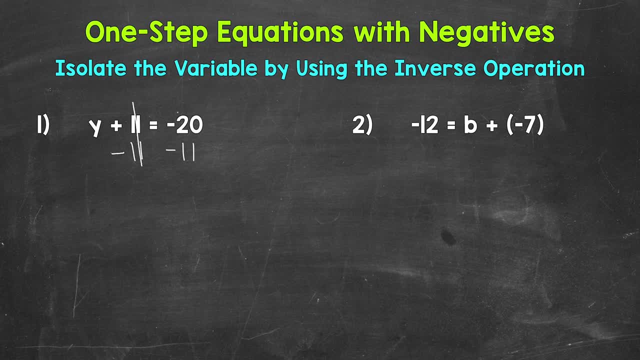 These 11s cancel each other out. They equal 0.. So y is now isolated. It's by itself y equals. Now, on the right side of the equation, we have negative 20 minus 11.. So we're starting with negative 20 and subtracting 11.. 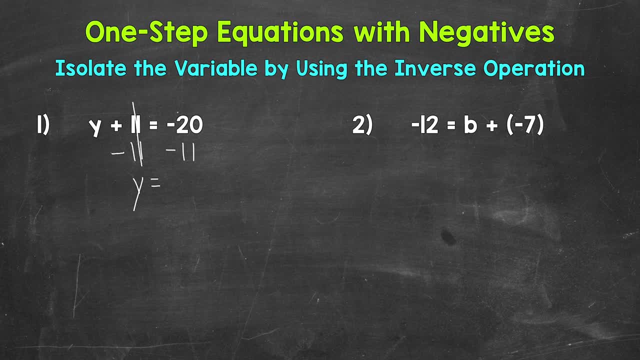 So we are decreasing in value by 11. We end up with negative 31. So y equals negative 31.. Now, one thing I do want to mention: it's always an option to come to the side in order to figure out a problem. 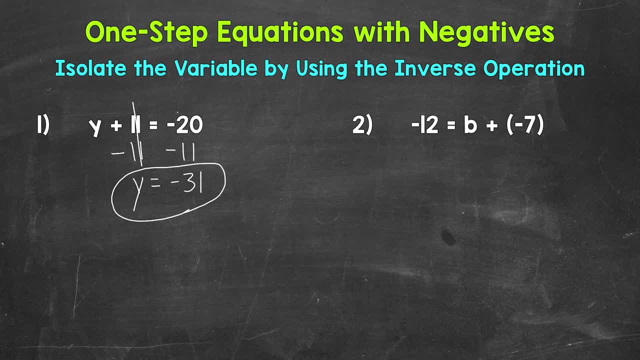 For example, negative 20 minus 11, we did vertically. You can come to the side and rewrite this horizontally if you prefer. Now, when we subtract, we can add the opposite. So let's add the opposite here. Add the opposite. 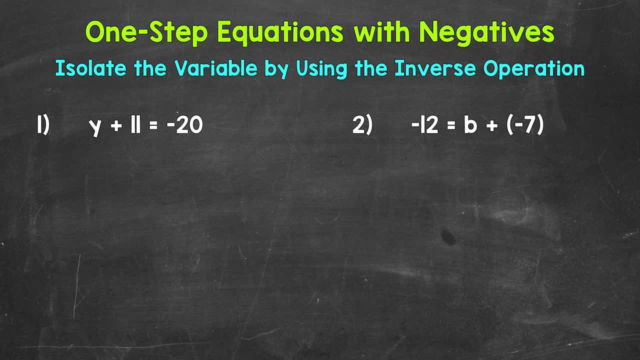 That way, the variable is by itself on one side of the equation. And again, we do this by using the inverse or opposite operation. Just remember: whatever is done to one side of the equation, it must be done to the other in order to keep everything balanced and equal. 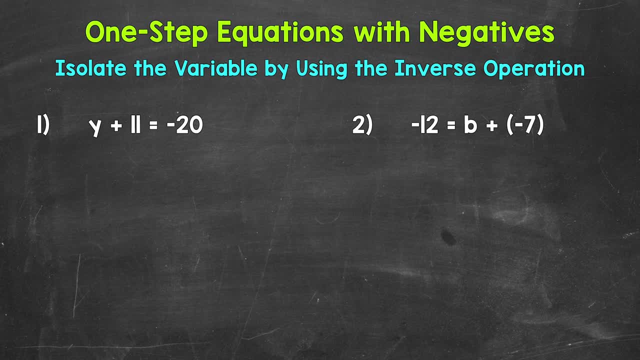 Let's jump into number one, where we have: y plus 11 equals negative 20.. Now we need to isolate that variable of y. We need to figure out what y equals. Since 11 is being added to y, we need to undo that addition by using the inverse operation. 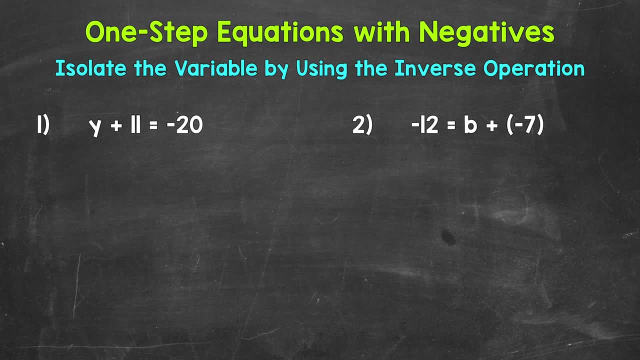 so the opposite operation, The other way around, The opposite of addition is subtraction. So let's subtract 11 from the left side of the equation. Now, whatever we do to one side of the equation, we must do to the other in order to keep it balanced and equal. 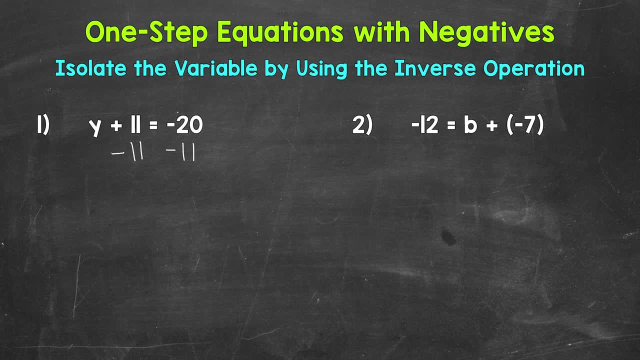 So let's subtract 11 from the right side as well. Now, if we take a look at the left side of the equation, we are adding 11 and subtracting 11.. So the opposite of addition is subtraction. So let's subtract 11 from the right side as well. 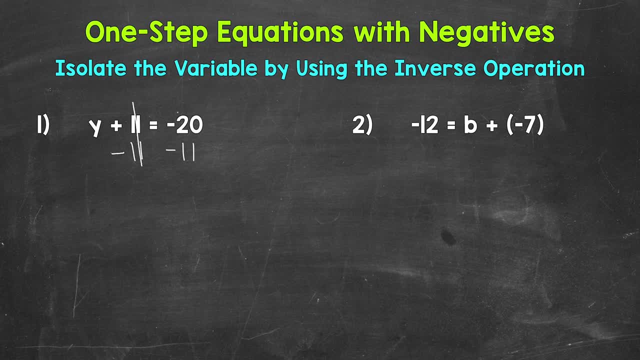 These 11s cancel each other out. They equal 0.. So y is now isolated. It's by itself y equals. Now, on the right side of the equation, we have negative 20 minus 11.. So we're starting with negative 20 and subtracting 11.. 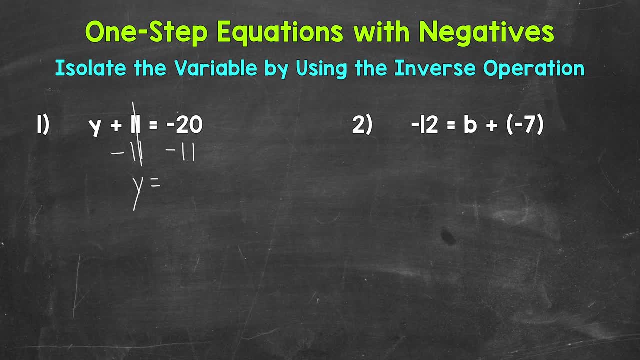 So we are decreasing in value by 11. We end up with negative 31. So y equals negative 31.. Now, one thing I do want to mention: it's always an option to come to the side in order to figure out a problem. 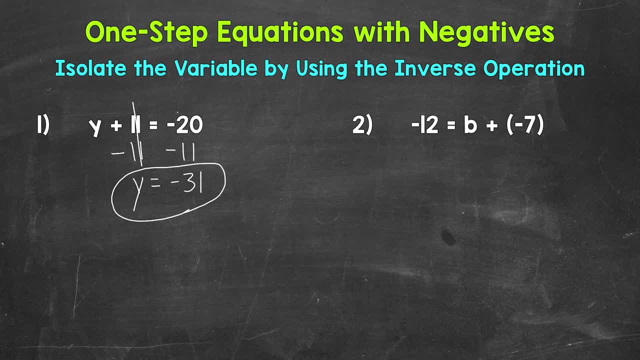 For example, negative 20 minus 11, we did vertically. You can come to the side and rewrite this horizontally if you prefer. Now, when we subtract, we can add the opposite. So let's add the opposite here. Add the opposite. 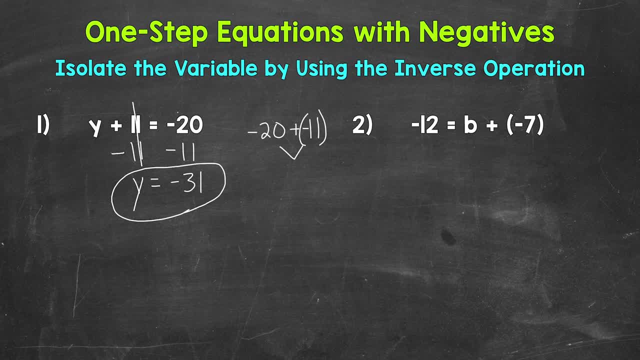 So negative 20 plus negative 11. Gives us that negative 31. So again, you can always come to the side to show work or set up a problem differently. So something to keep in mind. So our solution for number 1 is negative 31.. 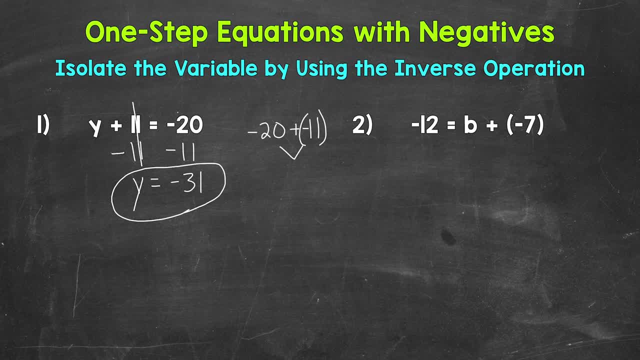 So negative 20 plus negative 11. Gives us that negative 31. So again, you can always come to the side to show work or set up a problem differently. So something to keep in mind. So our solution for number 1 is negative 31.. 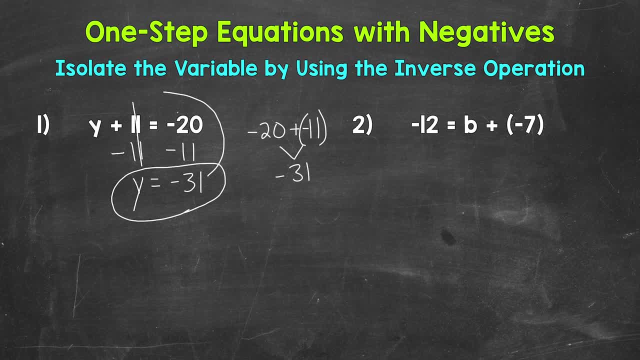 We can always check a solution by plugging it into the original equation. So let's plug negative 31 in for y and see if this works. Negative 31. Plus 11 equals negative 20.. So we're starting at negative 31 and adding 11.. 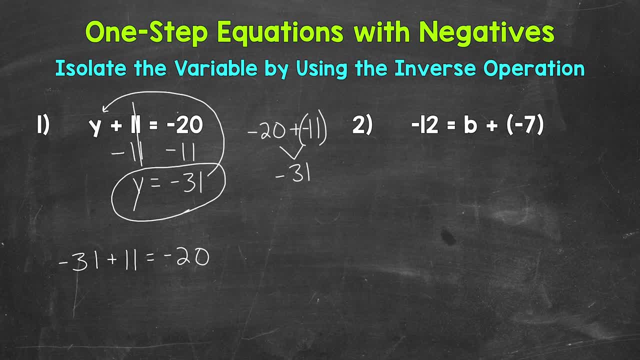 So we are increasing in value by 11.. Negative 31 plus 11 does equal negative 20. So we have the correct solution: y equals negative 31.. Let's move on to number 2, where we have negative 12 equals b plus negative 7.. 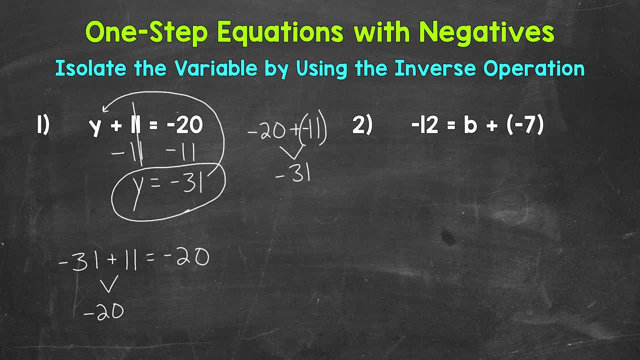 We need to isolate That variable of b. Negative 7 is being added to b, So we need to undo that addition by using the inverse operation. Let's subtract negative 7 from the right side. Whatever we do to one side of the equation, we must do to the other. 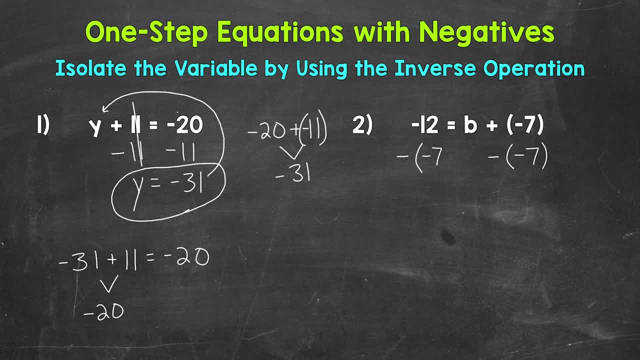 So let's subtract negative 7 from the left side as well. Now, if we take a look at the right side of the equation, we are adding a negative 7 and subtracting a negative 7.. These negative 7s are going to cancel out and equal 0.. 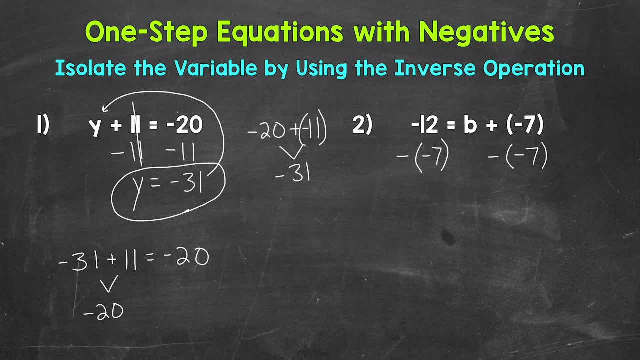 But it's kind of difficult to think through when we are subtracting a negative. When we subtract a negative, we actually increase in value And remember we can add the opposite. That's going to make this simpler to think through and see how the variable ends up isolated. 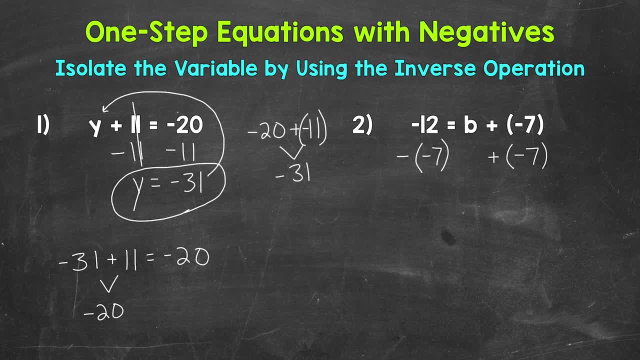 So let's add the opposite. Add And then the opposite of negative 7 is positive 7. So whenever we subtract a negative, we can add a positive. So now we have a negative 7 and a positive 7. These 7s cancel out. 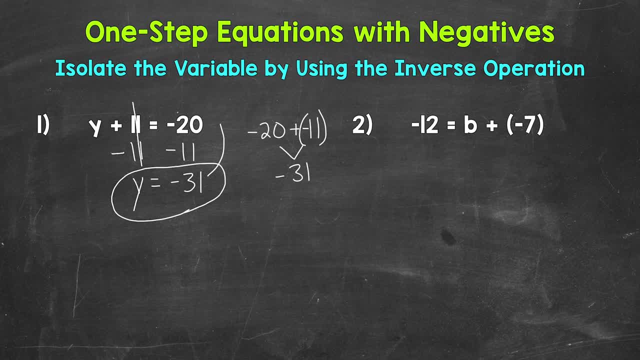 We can always check a solution by plugging it into the original equation. So let's plug negative 31 in for y and see if this works. Negative 31. Plus 11 equals negative 20.. So we're starting at negative 31 and adding 11.. 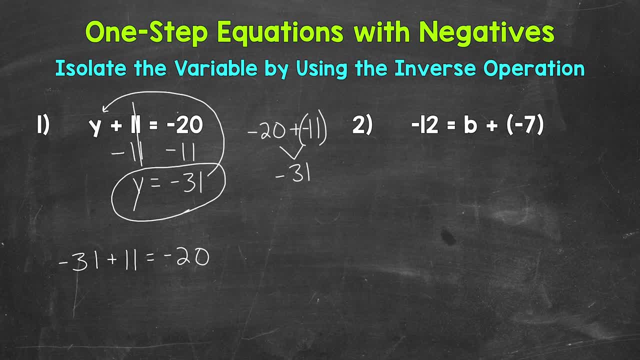 So we are increasing in value by 11.. Negative 31 plus 11 does equal negative 20. So we have the correct solution: y equals negative 31.. Let's move on to number 2, where we have negative 12 equals b plus negative 7.. 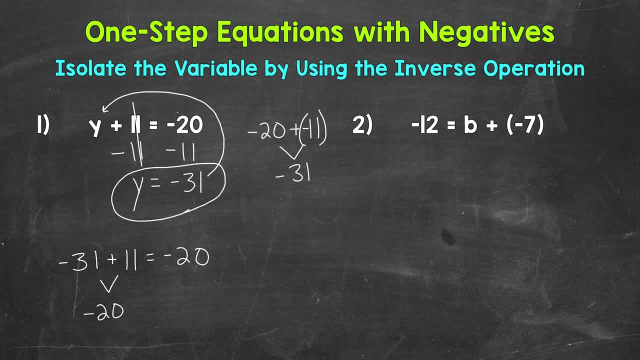 We need to isolate That variable of b. Negative 7 is being added to b, So we need to undo that addition by using the inverse operation. Let's subtract negative 7 from the right side. Whatever we do to one side of the equation, we must do to the other. 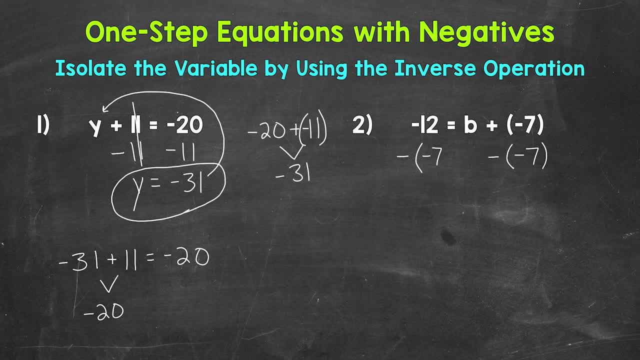 So let's subtract negative 7 from the left side as well. Now, if we take a look at the right side of the equation, we are going to see that the right side of the equation is the same as the left side. So we are adding a negative 7 and subtracting a negative 7.. 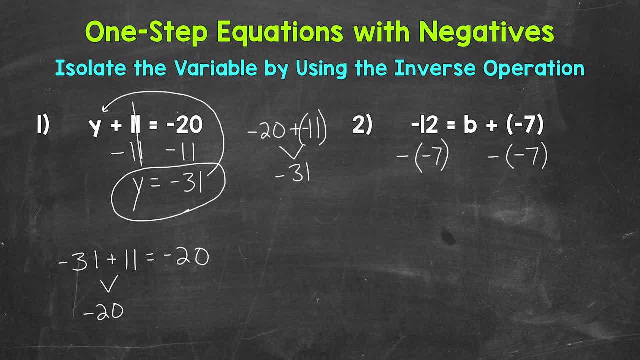 These negative 7s are going to cancel out and equal 0. But it's kind of difficult to think through when we are subtracting a negative. When we subtract a negative we actually increase in value And remember we can add the opposite. 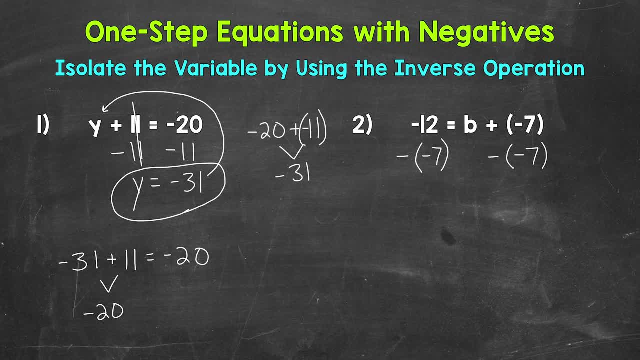 That's going to make this simpler to think through and see how the variable ends up isolated. So let's add the opposite. So when we subtract a negative we can add a positive. So now we have a negative 7 and a positive 7.. 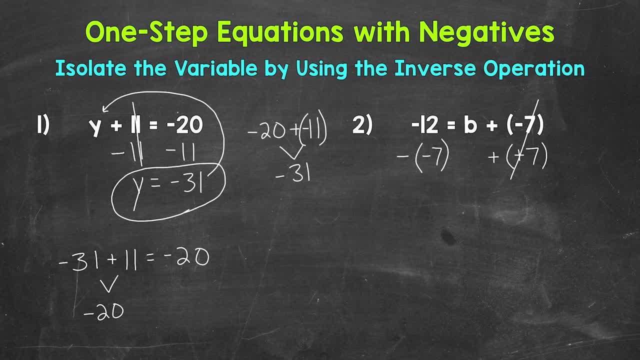 These 7s cancel out. They equal 0. So the variable is now isolated. b equals. And then on the left side we have negative 12 minus 0. Negative 7. Let's add the opposite. Add the opposite. 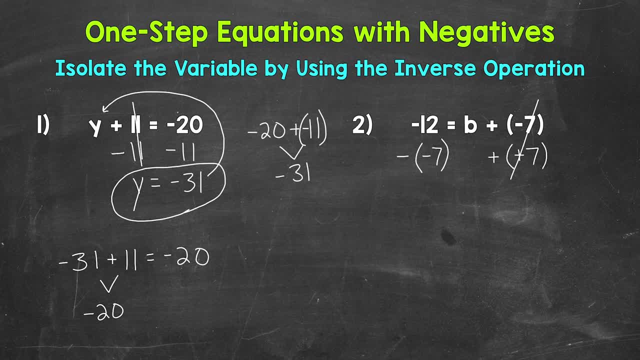 They equal 0. So the variable is now isolated. b equals. And then on the left side we have negative 12 minus negative 7.. Let's add the opposite. Add The opposite: Negative 12 plus a positive 7 equals negative 5.. 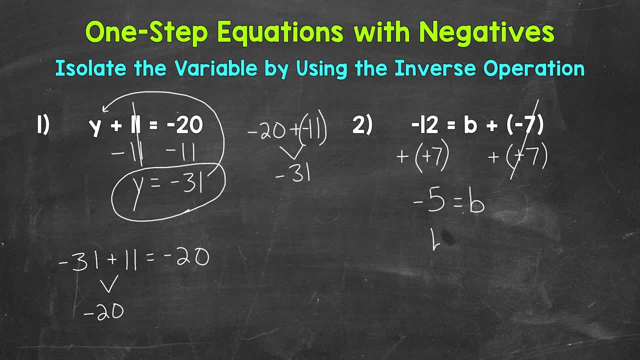 So b equals negative 5.. We can rewrite this with the variable coming first And remember we can always come to the side in order to show work or set up a problem differently. For example, Let's do negative 12 minus negative 7 off to the side and set it up horizontally. 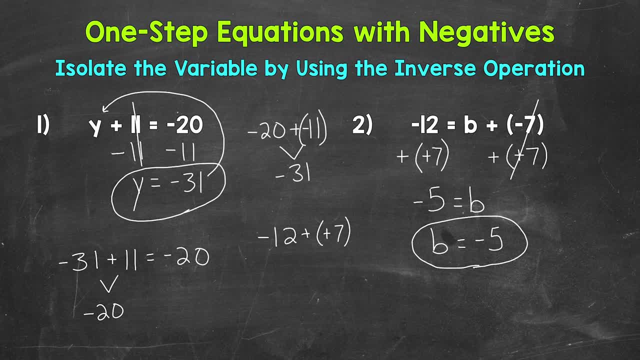 Let's add the opposite. So add the opposite: Negative 12 plus a positive 7 gives us negative 5.. Now let's check that solution of negative 5 and plug it in for b, So negative 12.. Equals: Negative 5 plus negative 7.. 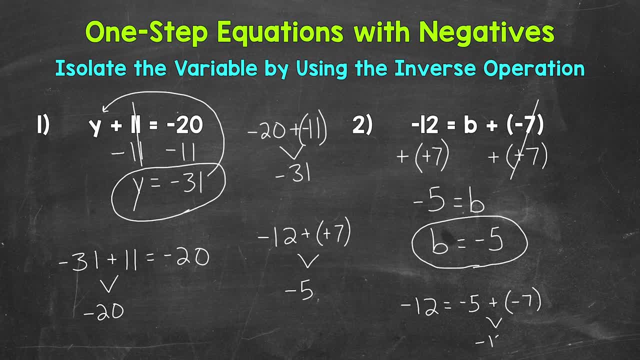 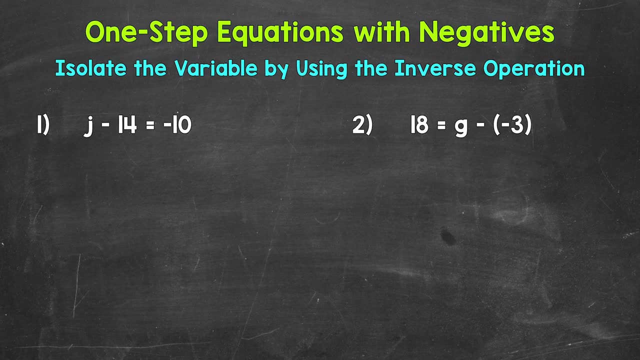 Negative 5 plus negative 7 does equal negative 12. So we have the correct solution: B equals negative 5.. There's how we solve one-step addition equations with negatives. Let's move on to subtraction. Here are our examples of one-step subtraction equations with negatives. 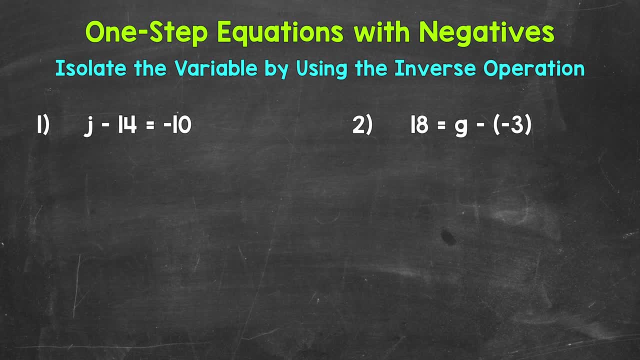 Let's move on to subtraction. Let's jump into number 1, where we have j minus 14 equals negative 10. We need to isolate that variable of j. We need to figure out what j equals. Since 14 is being subtracted from j, we need to undo that subtraction by using the inverse. 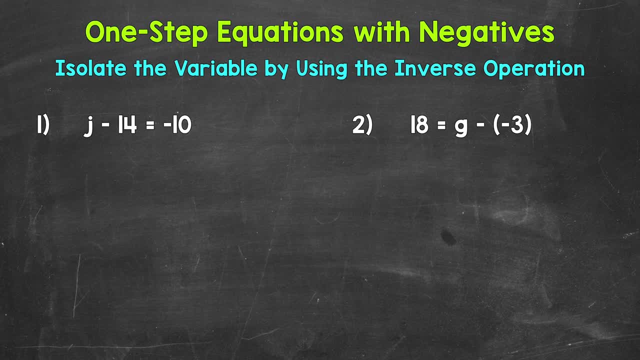 operation. So the opposite operation, The opposite of subtraction, is addition. So let's add 1. 14 to the left side of the equation. Now, whatever we do to one side of the equation, we must do to the other. So let's add 14 to the right side as well. 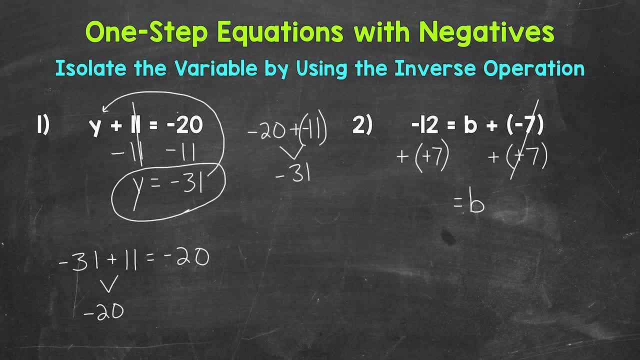 Negative 12 plus a positive 7 equals negative 5.. So b equals negative 5.. We can rewrite this with the variable coming first, And remember we can always come to the side in order to show work or set up a problem differently. 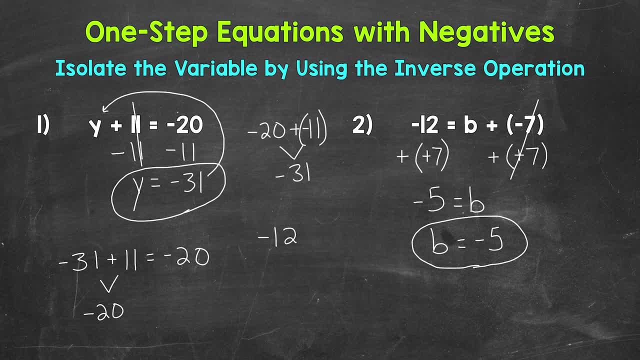 For example, let's do negative 12.. Negative 12 minus negative 7 off to the side and set it up horizontally. Let's add the opposite. So add the opposite. Negative 12 plus a positive 7 gives us negative 5.. 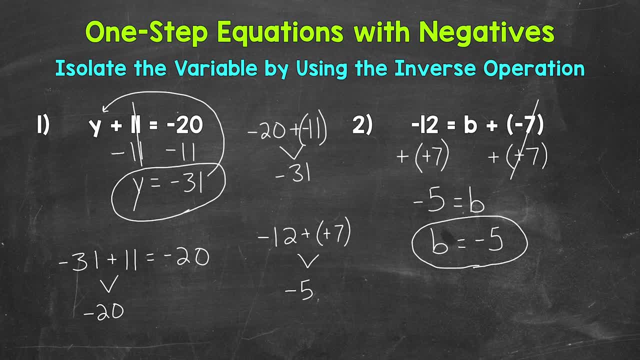 Now let's check that solution of negative 5 and plug it in for b. So negative 12 equals negative 5 plus negative 5.. So negative 12 plus a positive 7 gives us negative 5.. So negative 12 equals negative 5 plus a positive 7.. 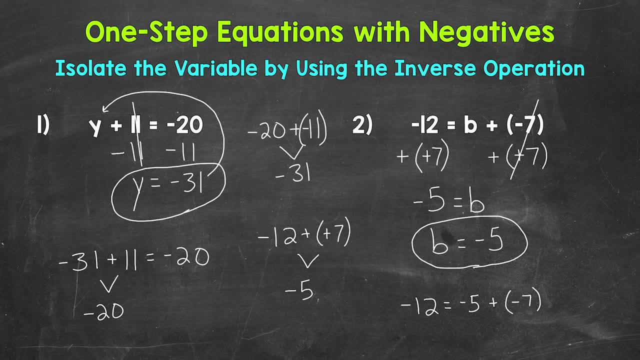 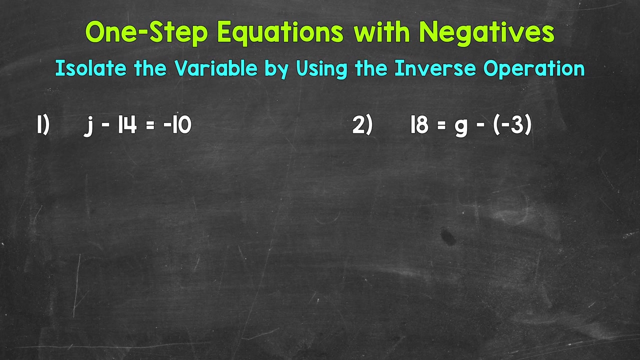 So we have the correct solution: b equals negative 5.. There's how we solve one-step addition equations with negatives. Let's move on to subtraction. Here are our examples of one-step subtraction equations with negatives. Let's jump into number 1, where we have 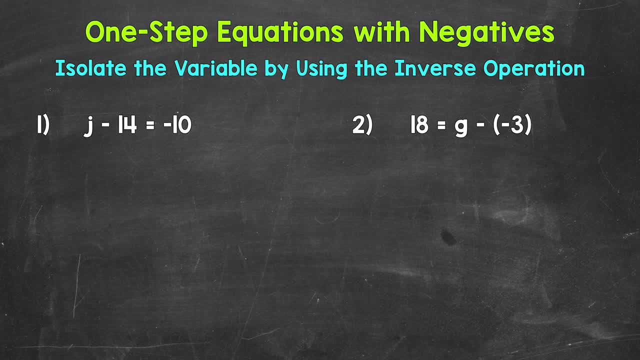 j minus 14 equals negative 10.. We need to isolate that variable of j. We need to figure out what j equals. Since 14 is being subtracted from j, we need to undo that subtraction by using the inverse operation, So the opposite operation. 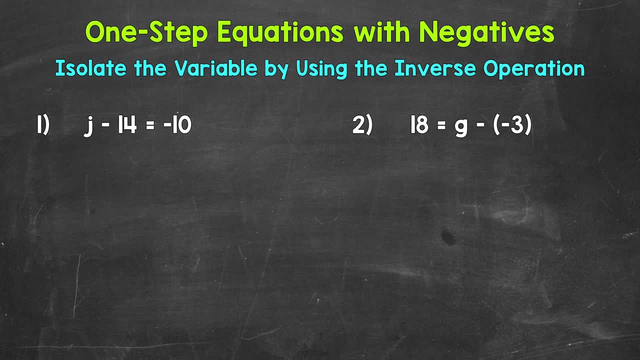 The opposite of subtraction is addition. So let's add 14 to the left. So let's add 14 to the right, So let's add 14 to the left side of the equation. Now, whatever we do to one side of the equation, we must do to the other. 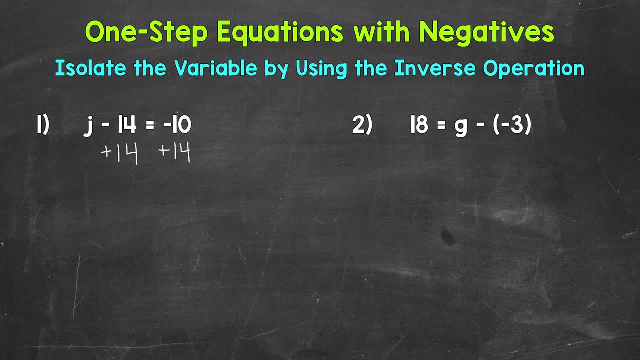 So let's add 14 to the right side as well. Now on the left side we are subtracting 14 and adding 14.. So these 14s cancel out. They equal 0.. The variable is now isolated. 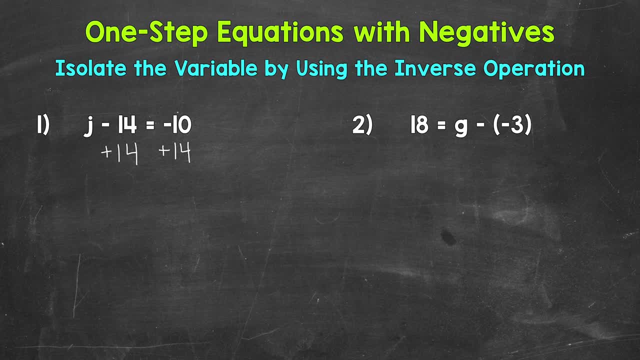 Now on the left side we are subtracting 14 and adding 14.. So these 14's cancel out. They equal 0.. The variable is now isolated. j is now by itself, So we have j equals. And then on the right side of the equation we have negative 10 plus 14.. 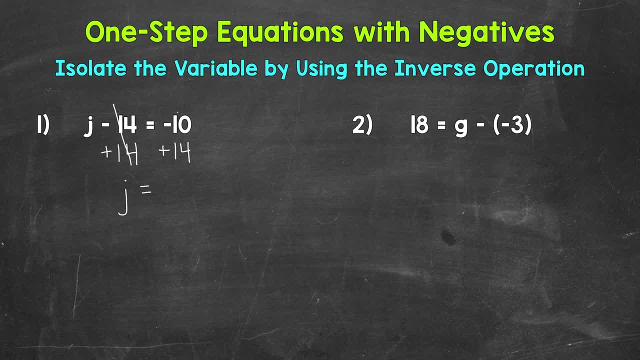 We are starting at negative 10 and increasing in value by 14. So we end up with positive 4.. j equals 4.. Now, one thing I do want to mention: We always have the option to come to the side in order to show work or set up a problem. 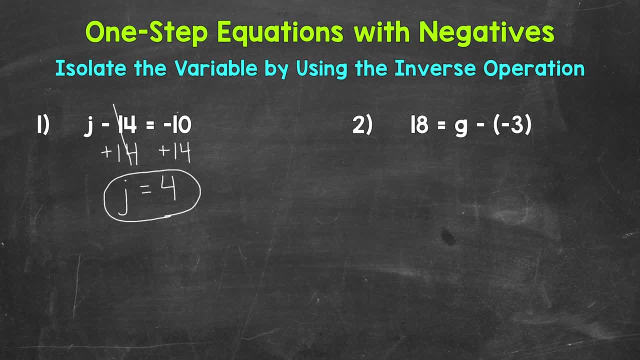 differently. For example, negative 10 plus 14. we solved vertically, so up and down. If you prefer to work through that horizontally, you can always rewrite the problem off to the side. So negative 10 plus 14. That equals 4.. 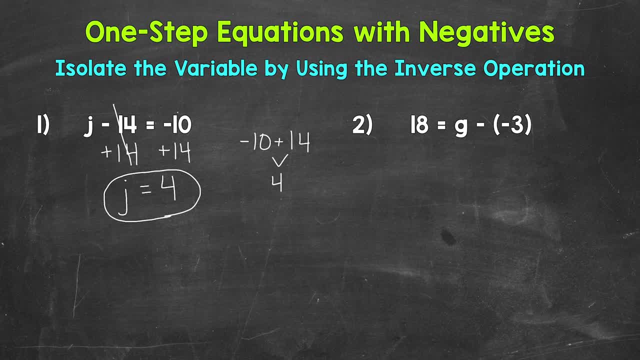 So you always have that option. Now, j equals 4.. That's our solution. We can always check a solution and make sure it works. So let's plug 4 into the original equation. So let's plug 4 in for j and see if this works. 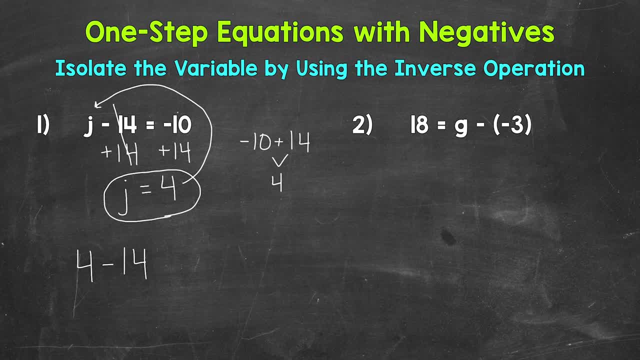 So 4 minus 14 equals negative 10.. 4 minus 14 does equal negative 10.. So we have the correct solution: j equals 4.. Let's move on to number 2, where we have 18 equals g minus 14.. 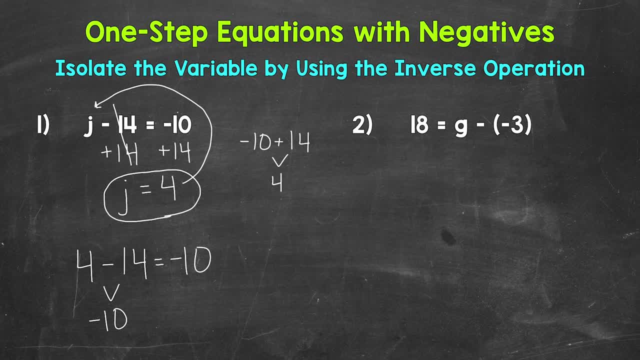 So we have the correct solution: j equals 4.. And because 28 equals 1 minus 4, downhill goes beyond 34ฅ, we cancel it by 36.. 29 equals 40. And because 28 equals 4 is Pan without 보면, which is 1 if you press play at page 4.. 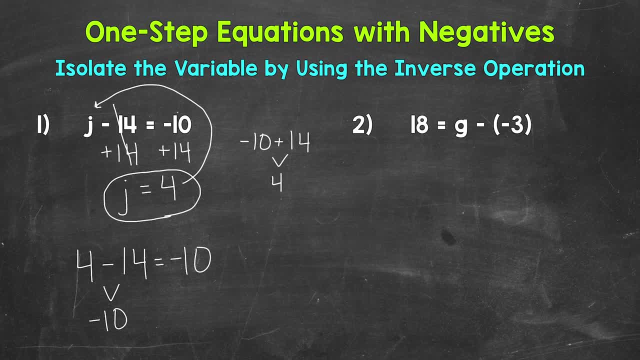 We approve, We must cancel it. It's OK Because i Is equal to 3 minus –3,. we need to isolate that variable of g. Negative 3 is being subtracted from g. We need to undo that subtraction by using the inverse operation. 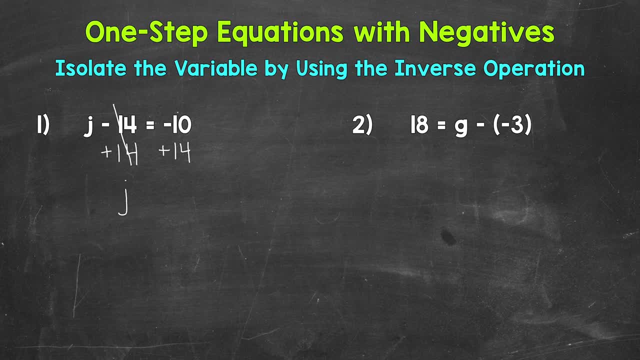 j is now by itself. So we have: j equals negative 10.. So we have: j equals negative 10.. J equals. And then on the right side of the equation, we have negative 10 plus 14. We are starting at negative 10 and increasing in value by 14.. 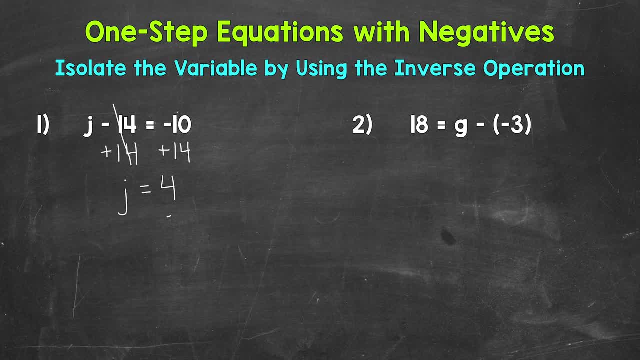 So we end up with positive 4.. j equals 4.. Now, one thing I do want to mention: we always have the option to come to the side in order to show work or set up a problem differently. For example, negative 10 plus 14.. 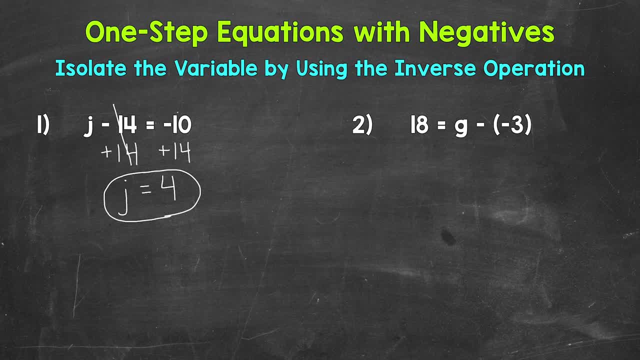 Come to the side 14. we solved vertically, so up and down. if you prefer to work through that horizontally, you can always rewrite the problem off to the side. so negative: 10 plus 14, that equals 4, so you always have that option. now j equals 4. that's our solution. we can always check a solution and 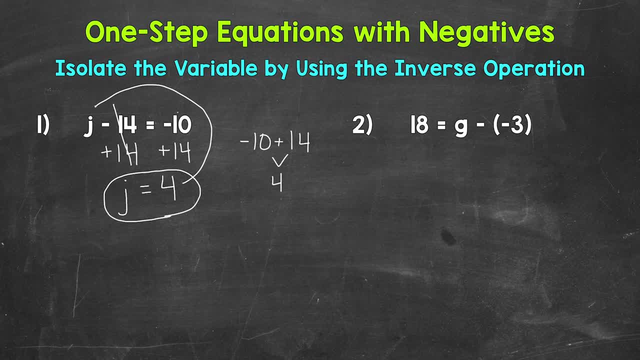 make sure it works by plugging it into the original equation. so let's plug 4 in for j and see if this works. so 4 minus 14 equals negative 10. 4 minus 14 does equal negative 10. so we have the correct solution: j equals 4. let's move on to number 2, where we have 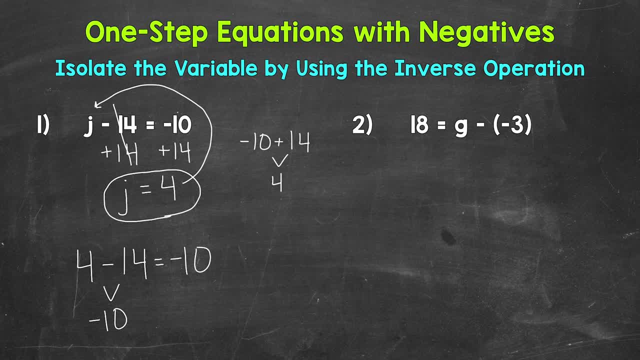 18 equals g minus negative 3. we need to isolate that variable of g. negative 3 is being subtracted from g. we need to undo that subtraction by using the inverse operation. the inverse of subtraction is addition. so let's add negative 3 to the right side of the equation. whatever we 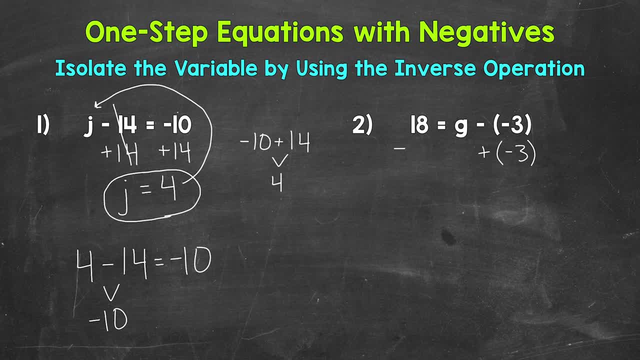 do to one side, we must do to the other. so let's add negative 3, so to the left side as well. let's take a look at the right side of the equation now. when we subtract a negative, we are actually increasing in value. so we are increasing g's value by 3. so by adding 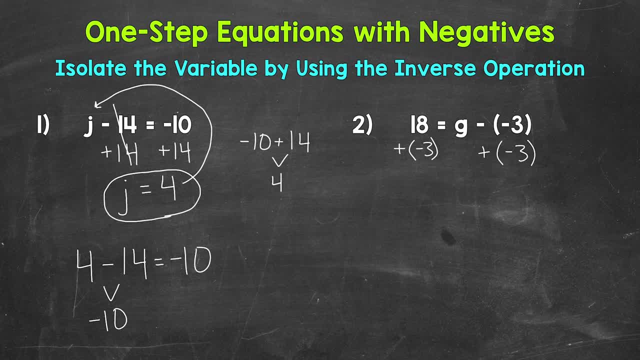 The inverse of subtraction is addition- left side as well. let's take a look at the right side of the equation now. when we subtract a negative, we are actually increasing in value. so we are increasing G's value by 3. so by adding negative 3 to that side of the equation, these 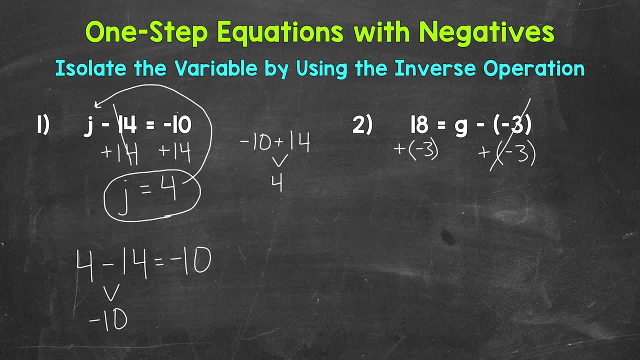 cancel out and equals 0. so our variable of G is now isolated. so G equals. and then on the left side of the equation, 18 plus negative 3 equals 15. so G equals 15 and we can rewrite that with the variable coming first. now, if we look, 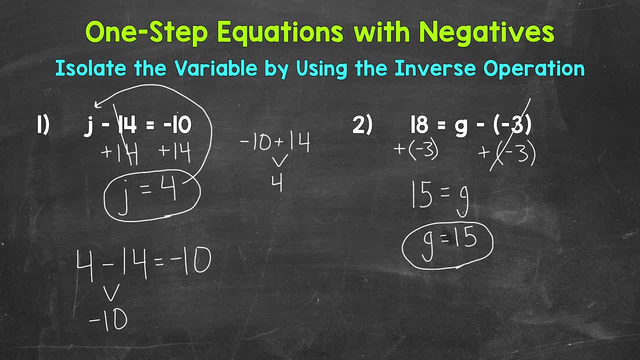 back up at the side of the equation. that can be a little confusing to think through because it looks like we have negative 3 plus negative 3, which would equal negative 6, not that 0 which isolated our variable. But keep in mind, when we subtract a negative, we increase in value, So g is increasing. 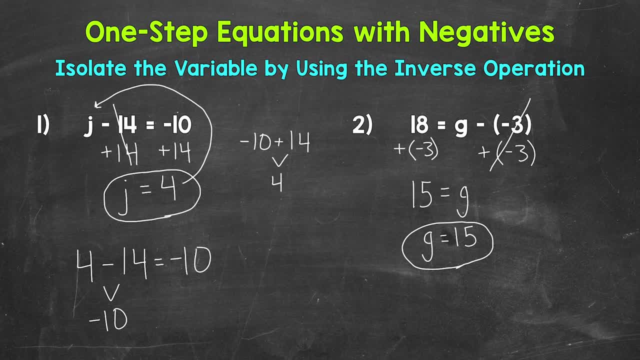 in value by 3.. By adding a negative 3 to that side of the equation, we are canceling that increase out to equal 0, and our variable was isolated. Here is an easier way to think about it: Whenever we subtract a negative, we can think of this as adding a positive And remember. 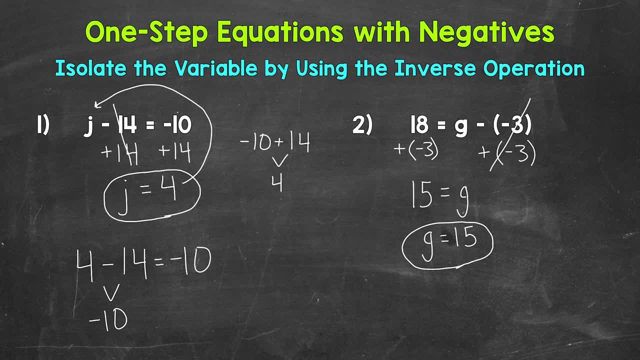 when subtracting we can always add the opposite. so this works out. We can actually rewrite this as: 18 equals g plus 3, g plus a positive 3, because again we can add the opposite. So add and then the opposite of negative 3 is positive 3.. So you can always rewrite the equation if you. 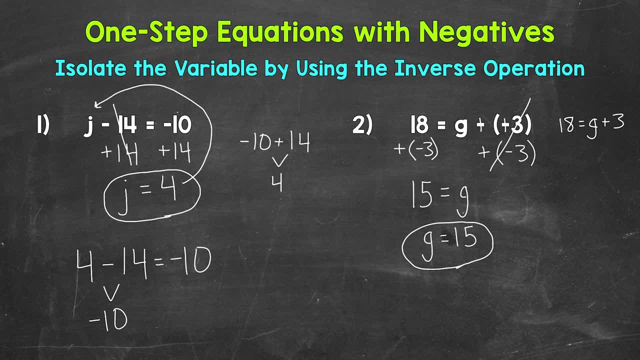 are subtracting a negative to add a positive. Let's go through the rewritten equation and see if we still get 15.. We need to isolate g. 3 is being added to g, so let's undo that addition by using the inverse operation, which is subtraction. Let's subtract 3 from the right side of the equation. Whatever we 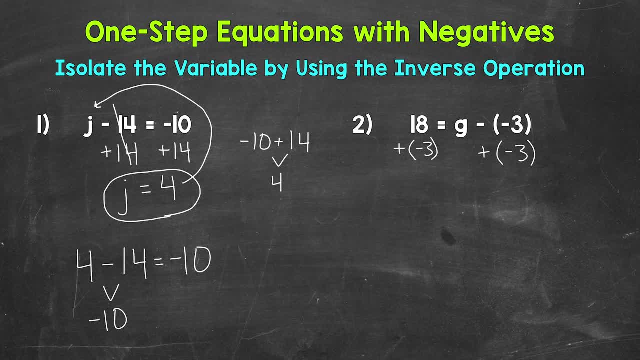 negative 3 to that side of the equation. these cancel out and equal 0. so our variable of g is now isolated. so g equals and then on the left side of the equation equals 15: 0. we can rewrite that with the variable 0: 0. 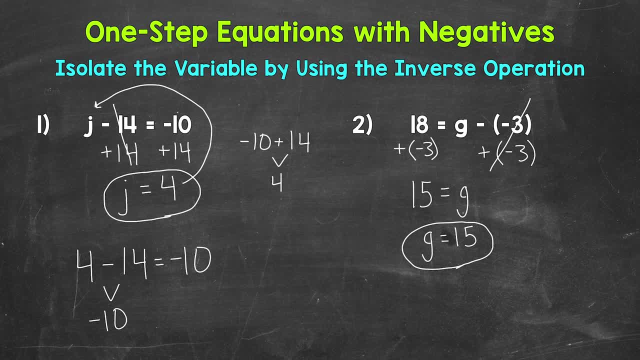 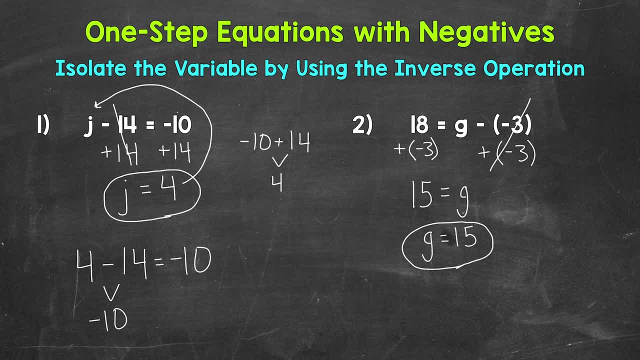 So g is increasing in value by 3.. By adding a negative 3 to that side of the equation, we are canceling that increase out to equal 0, and our variable was isolated. Here is an easier way to think about it. 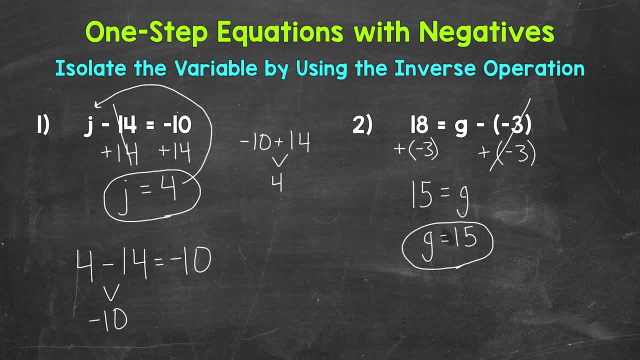 Whenever we subtract a negative, we can think of this as adding a positive And remember, when subtracting we can always add the opposite. So this works out. We can actually rewrite this as 18 equals g plus 3.. g plus a positive 3.. 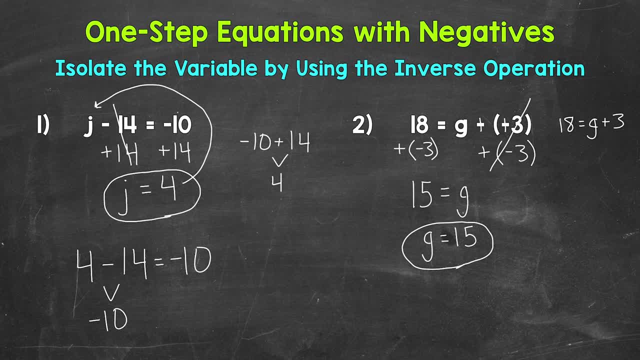 Because again, we can add the opposite. So add and then the opposite of negative 3. So you can always rewrite the equation if you are subtracting a negative to add a positive. Let's go through the rewritten equation and see if we still get 15.. 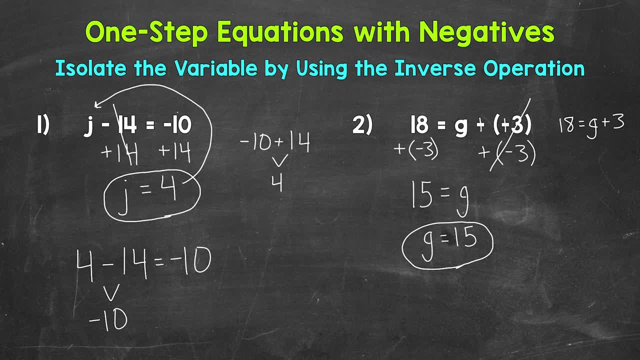 We need to isolate g. 3 is being added to g, so let's undo that addition by using the inverse operation, which is subtraction. Let's subtract 3 from the right side of the equation. Whatever we do to one side, we must do to the other. 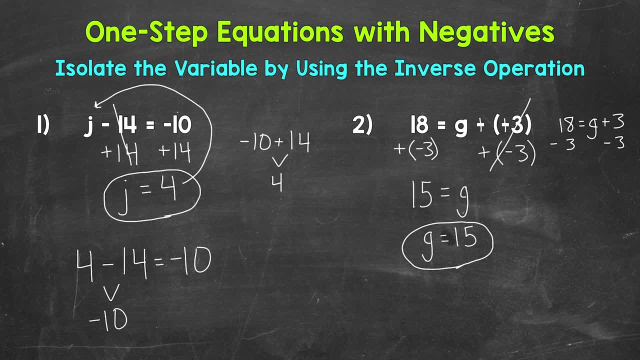 So subtract 3 from the left side as well. On the right side we are adding 3 and subtracting 3.. So these 3s cancel out. g is now isolated. So g equals, and then on the left side, 18 minus 3, that equals 15.. 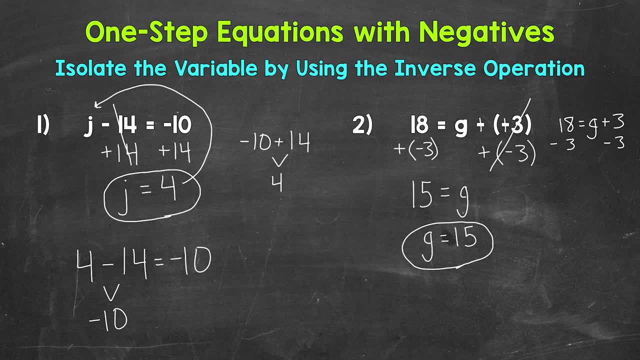 do to one side, we must do to the other. so subtract 3 from the left side as well. On the right side we are adding 3 and subtracting 3, so these 3s cancel out. So g equals. and then on the left side, 18 minus 3, that equals 15.. So g equals 15. that way. 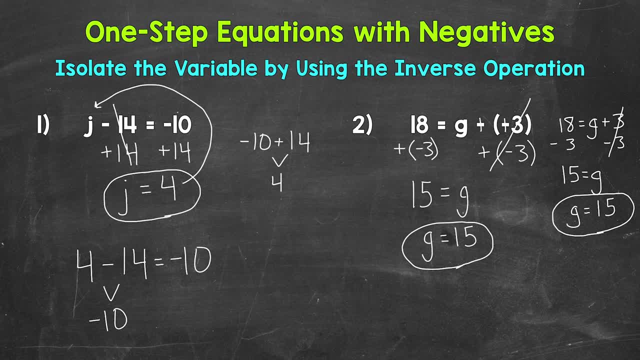 as well, And I do want to mention one more time that we can always come to the side in order to show work or set up a problem differently. For example, let's do 18 plus negative 3, horizontally, so side to side, 18 plus negative 3.. 18 plus negative 3 equals 15.. Let's check. 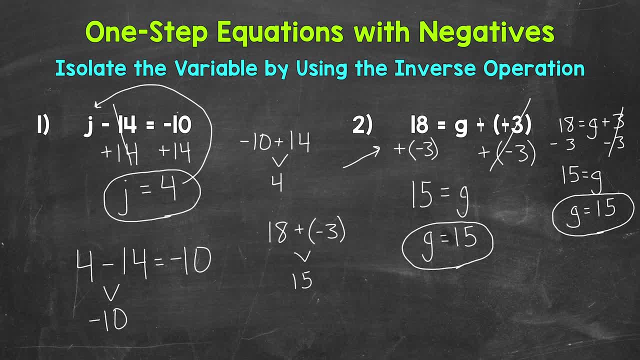 that solution of 15 by plugging 15 in for g in the original equation and see if this works. So we have: 18 equals 15 minus negative 3.. Since we are subtracting a negative, we are increasing the value. 15 minus negative 3 does equal 18, and we can always add the opposite. So add and then. 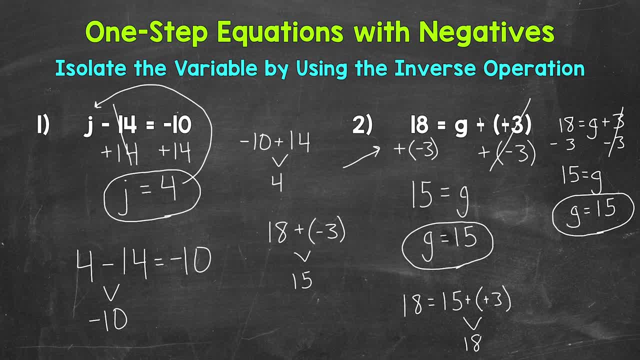 the opposite of negative 3 is positive 3.. So 15 plus positive 3 gives us 18 as well. We have the correct solution: g equals 15.. So there's how we solve one-step subtraction equations. Let's move on to multiplication. 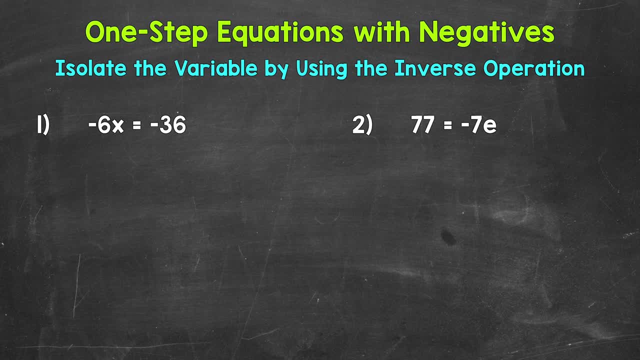 Our examples of one-step multiplication equations with negatives. Let's jump into number one, where we have negative 6x equals negative 36.. Now we have a number next to a variable. That means we are multiplying. This is negative. 6 times x equals negative 36.. So whenever you see a number next to 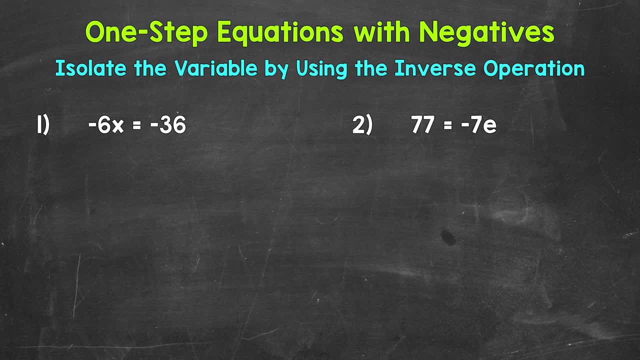 a variable that is representing multiplication. So something to keep in mind. Now we need to isolate that variable of x. We need to figure out what x equals. Since x is being multiplied by negative 6, we need to undo that multiplication by using the inverse operation. 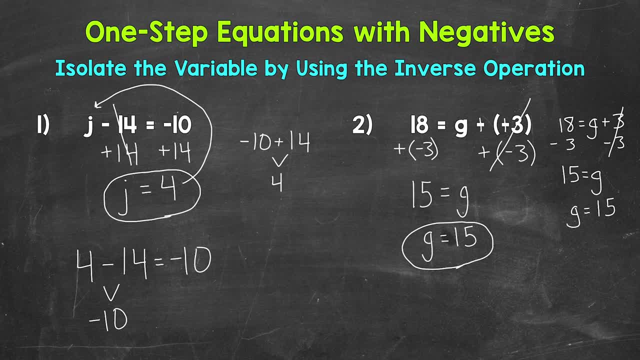 So g equals 15 that way, And I do want to mention one more time that we can always come to the side in order to show work or set up a problem differently. For example, let's do 18 plus negative 3 horizontally. 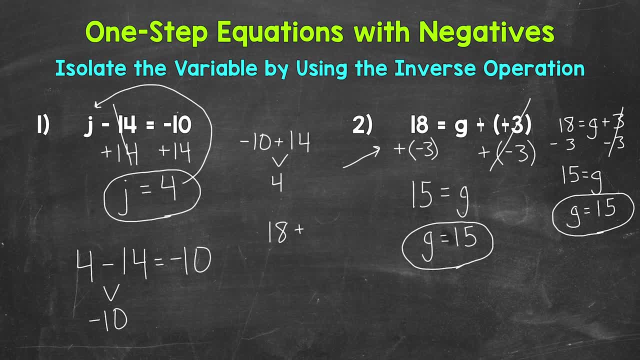 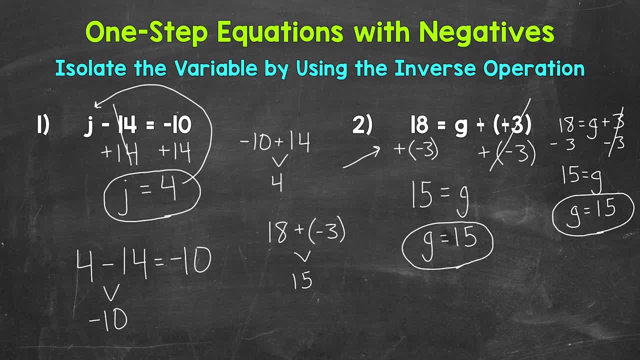 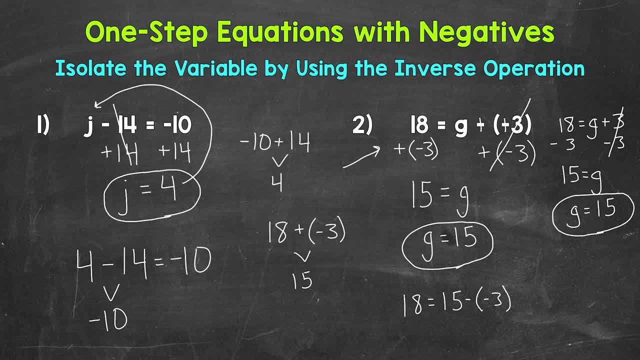 Since we are subtracting a negative, we are increasing in value. 15 minus negative 3 does equal 18.. And we can always add the opposite. So add and then the opposite of negative 3 is positive 3.. So 15 plus positive 3 goes to g. 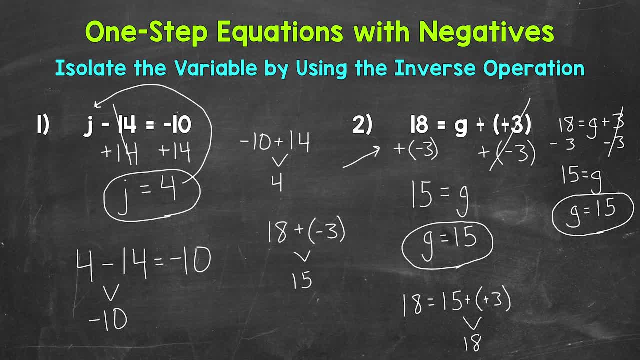 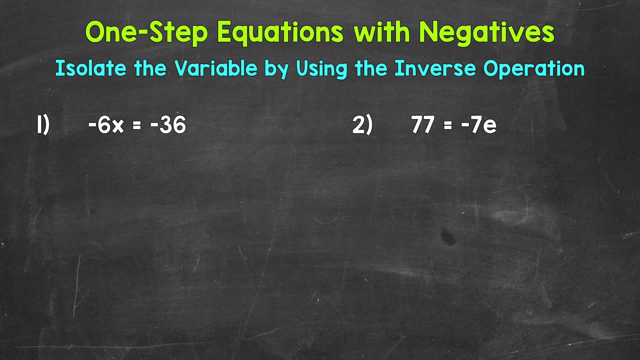 It gives us 18 as well. We have the correct solution: g equals 15.. So there's how we solve one-step subtraction equations. Let's move on to multiplication. So here are our examples of one-step multiplication equations with negatives. Let's jump into number one, where we have negative 6x equals negative 36.. 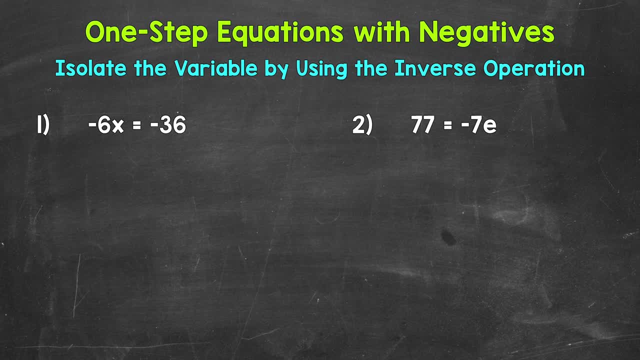 Now we have a number next to a variable. That means we are multiplying. This is negative. 6 times x equals negative 36. So whenever you see a number next to a variable, that is representing multiplication. So something to keep in mind. 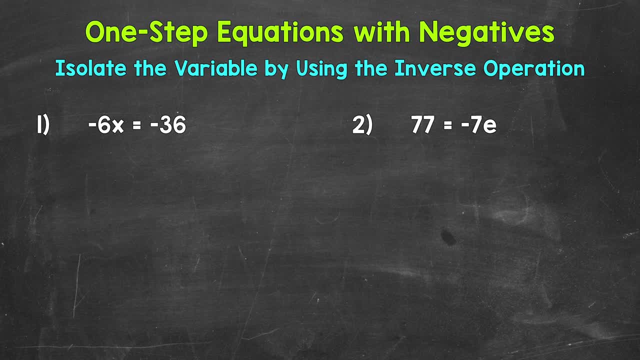 Now we need to isolate that variable of x. We need to figure out what x equals. Since x is being multiplied by negative 6, we need to undo that multiplication by using the inverse operation. So the opposite operation, The opposite of multiplication, is division. 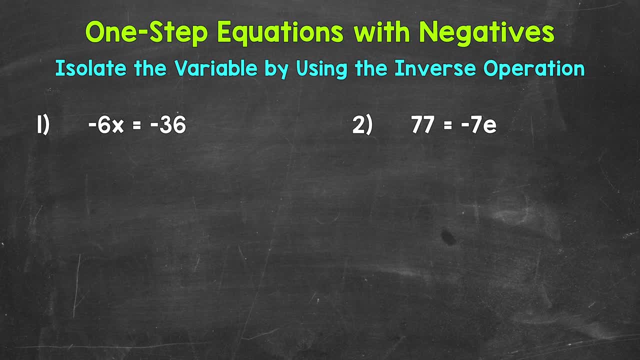 So the opposite operation, The opposite of multiplication, is division. So let's divide the left side of the equation by negative 6.. Whatever we do to one side of the equation, we must do to the other in order to keep it balanced and equal. So let's divide the right. 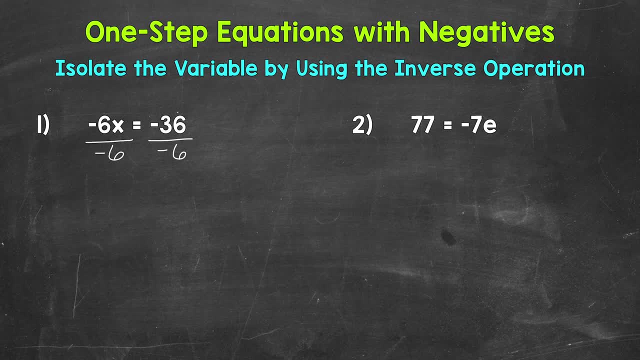 side, by negative 6 as well. Now let's take a look at the left side of the equation. We are multiplying by negative 6 and dividing by negative 6.. So these negative 6s cancel out. They equal a positive 1, because we have negative 6 divided by negative 6, a negative divided by a. 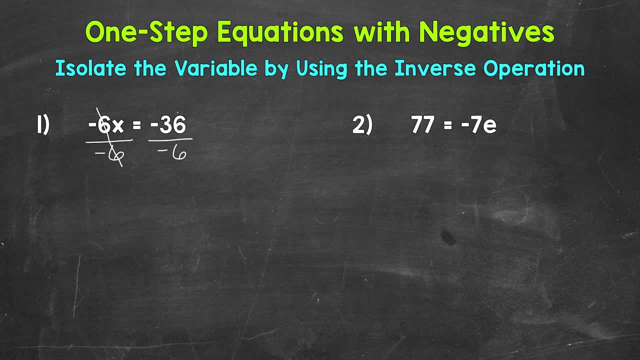 negative equals a positive, So we end up with a positive 1. This gives us 1x, which is just x. So x is now isolated. It's by itself x equals. and then on the right side of the equation, 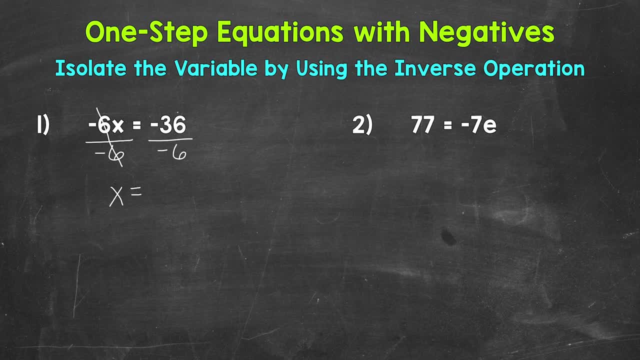 negative, 36 divided by negative, 6 equals a positive 6. Because, again, a negative divided by a negative equals a positive. So this is our solution: x equals 6.. Now we can always check a solution by plugging it into the original equation. 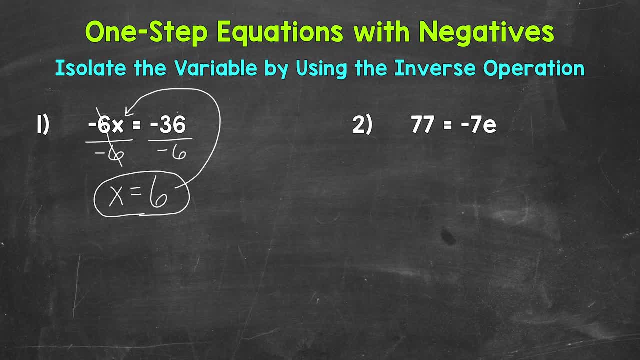 So let's plug 6 in for x and see if this works. So we have negative 6 times a positive, 6 equals negative, 36.. A negative times a positive equals a negative. So negative 6 times a positive 6 does equal negative. 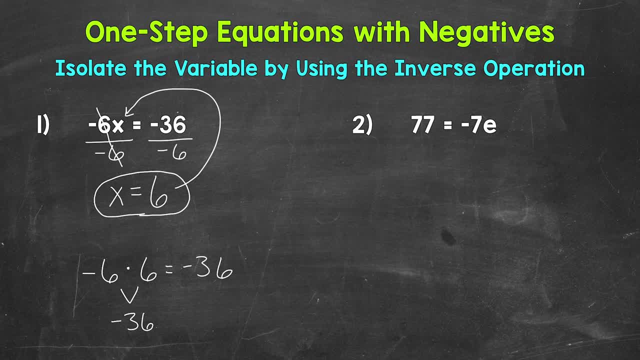 We have the correct solution: x equals 6.. Let's move on to number 2, where we have 77 equals negative 7e. So we need to isolate that variable of e. e is being multiplied by negative 7. We need to undo that multiplication by using the inverse operation, The inverse of multiplication. 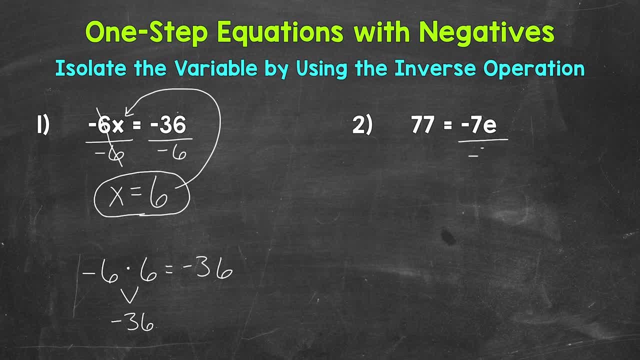 is division. So let's divide the right side by negative 7.. So we have negative 7 divided by negative 7.. Whatever we do to one side of the equation, we must do to the other. So let's divide the left side by negative 7 as well. Now, taking a look at the right side of the equation, we are multiplying. 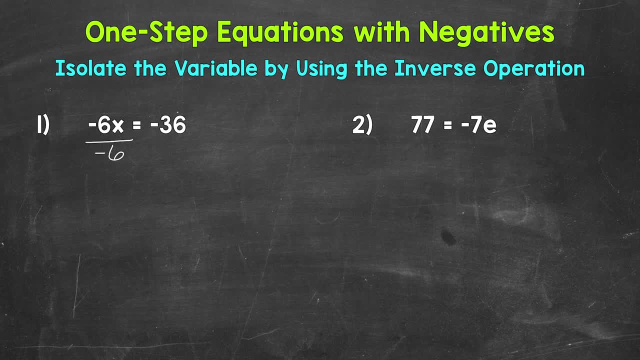 So let's divide the left side of the equation by negative 6.. Whatever we do to one side of the equation, we must do to the other in order to keep it balanced and equal. So let's divide the right side by negative 6 as well. 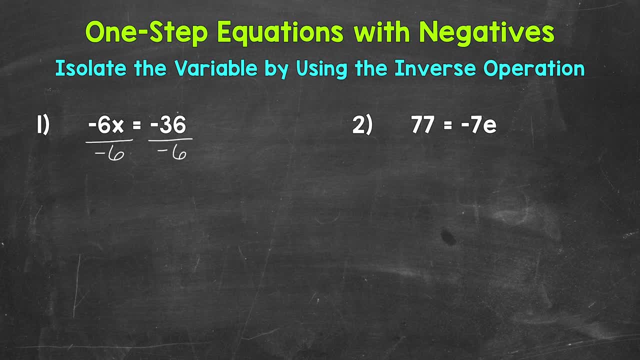 Now let's take a look at the left side of the equation. We are multiplying by negative 6 and dividing by negative 6. So these negative 6s cancel out. They equal a positive 1, because we have negative 6 divided by negative 6.. 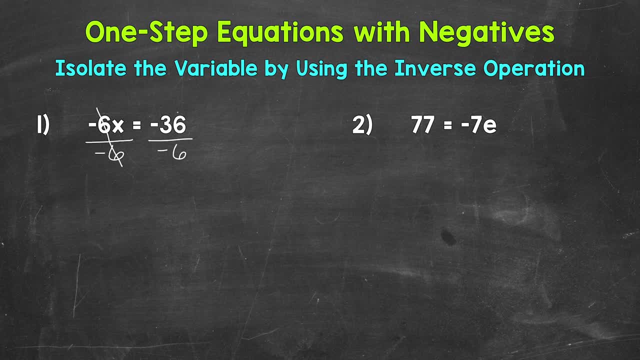 A negative divided by a negative equals a positive, So we end up with a positive 1. This gives us 1x, which is just x. So x is now isolated. It's by itself x, x equals. And then, on the right side of the equation, negative 36 divided by negative 6 equals a. 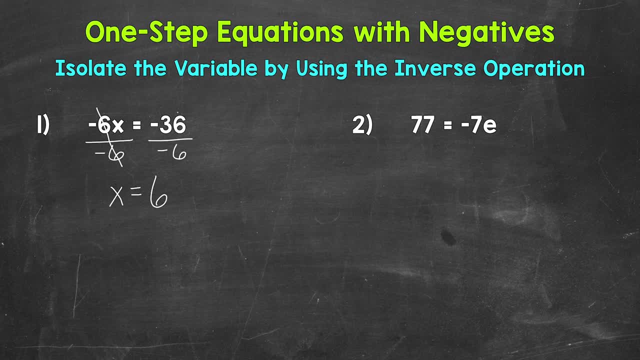 positive 6. Because, again, a negative divided by a negative equals a positive. So this is our solution: x equals 6.. Now we can always check a solution by plugging it into the original equation. So let's plug 6 in for x and see if this works. 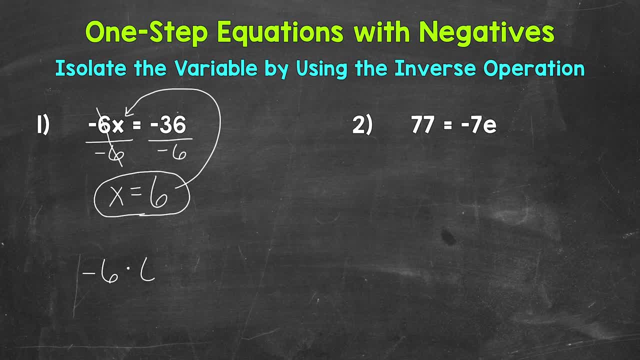 So we have negative 6 times a positive: 6 equals negative 36.. A negative times a positive equals a negative. So negative 6 times a positive 6 does equal negative 36.. We have the correct solution: x equals 6.. 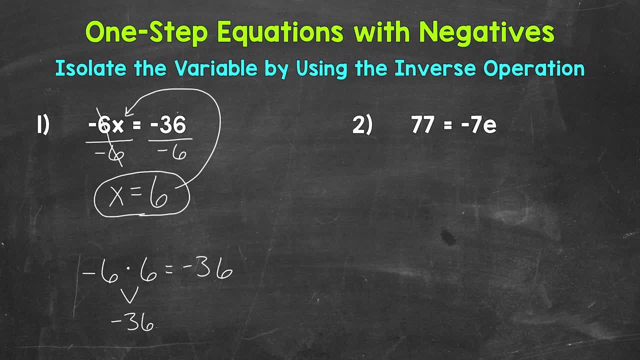 Let's move on to number 2, where we have 77 equals negative 7e. So we need to isolate that variable of e. e is being multiplied by negative 7. We need to undo that multiplication by using the inverse operation. The inverse of multiplication is division. 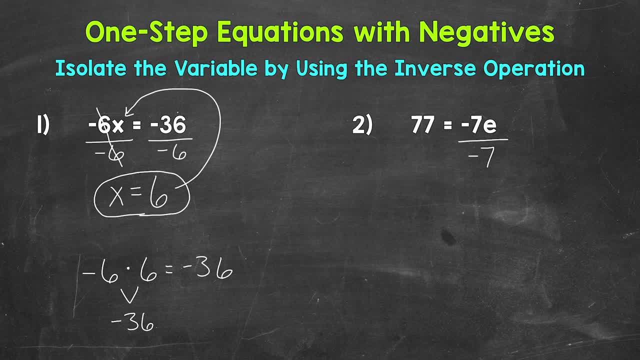 So let's divide the right side by negative 7.. Whatever we do to one side of the equation, we must do to the other, So let's divide the left side by negative 7 as well. Now, taking a look at the right side of the equation, we can see that the left side is: 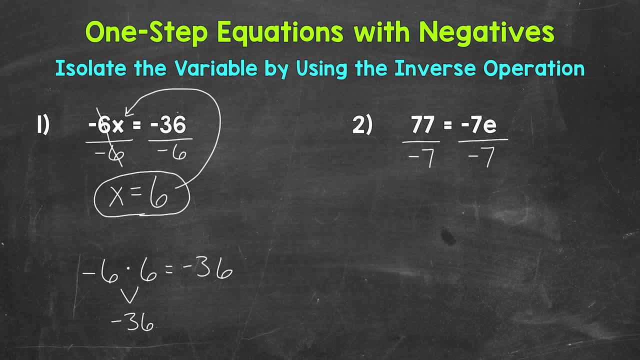 divided by negative 7.. On the right side of the equation we are multiplying by negative 7 and dividing by negative 7. So these negative 7s cancel out. They equal 1. We have negative 7 divided by negative 7.. 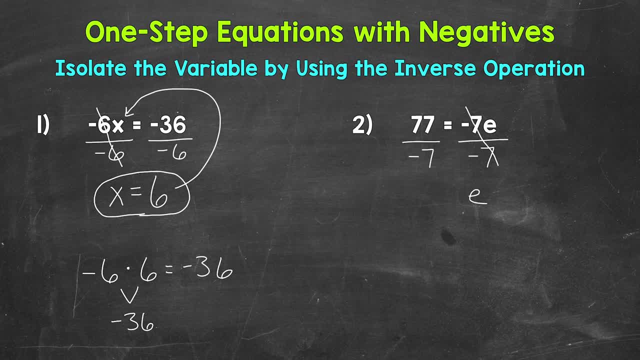 That gives us 1e, which is just e. Our variable is now isolated. It's by itself e equals. and then, on the left side of the equation, we have 77 divided by negative 7. So a positive divided by a negative. 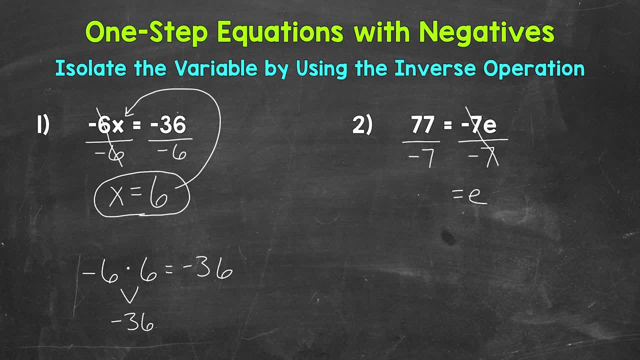 That's going to equal a negative, So we get negative 11.. e equals negative 11.. And we can rewrite this with the variable coming first. So e equals negative 11.. Let's check that solution by plugging negative 11 in for e. 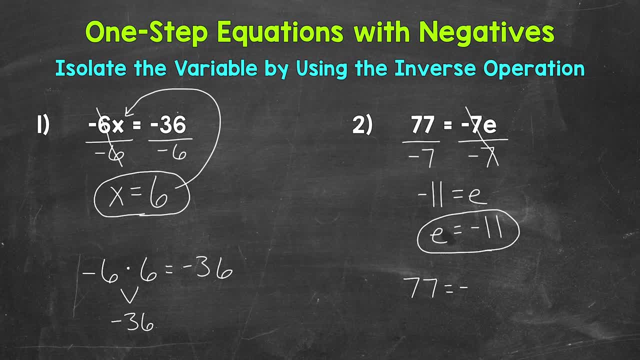 So we have 77 equals negative, 7 times negative, 11.. We have a negative times a negative, Negative, 7 times negative, 11.. A negative times a negative equals a positive. So negative 7 times negative, 11 does equal 77.. 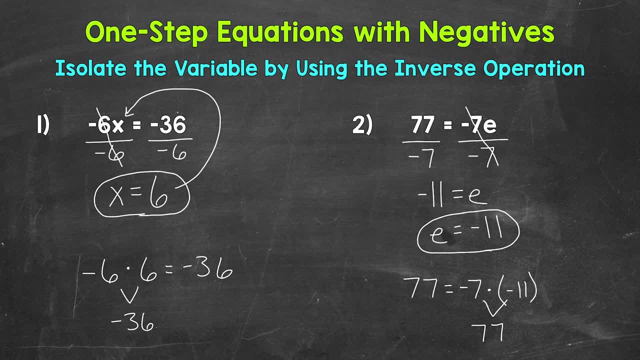 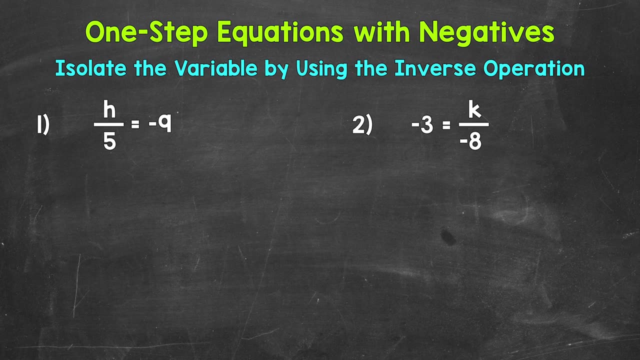 A positive 77.. We have the correct solution: e equals negative 11.. There's how we solve one-step multiplication equations with negatives. Let's move on to division. Here are our examples of one-step division equations with negatives. Let's jump into number 1, where we have: h divided by 5 equals negative 9.. 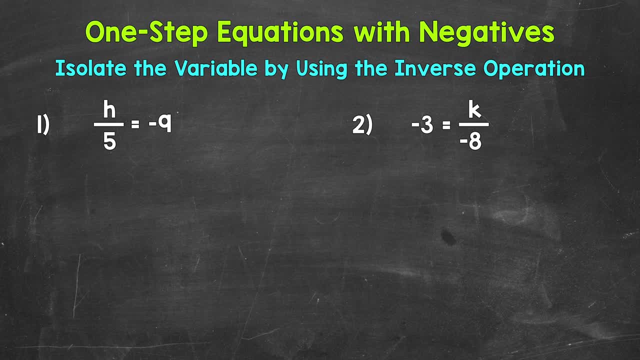 Now we need to isolate that variable of h. We need to figure out what h equals. Since h is being divided by 5, we need to undo that division by using the inverse. So the opposite operation, the opposite of division, is multiplication. 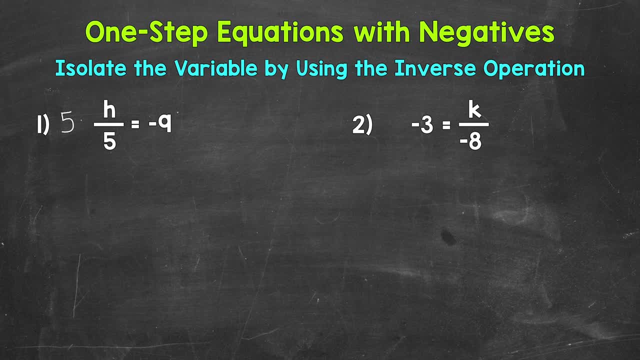 So let's multiply the left side of the equation by 5.. Now, whatever we do to one side of the equation, we must do to the other in order to keep it balanced and equal. Let's multiply the right side of the equation by 5 as well. 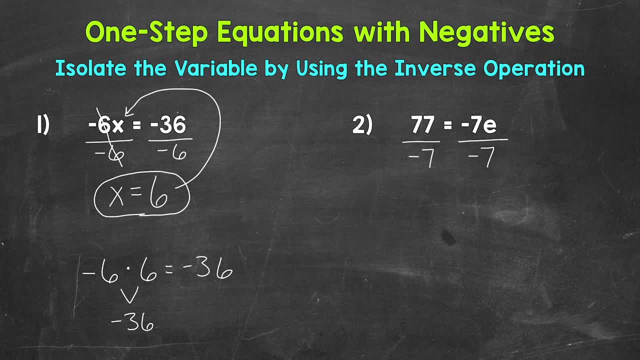 by negative 7 and dividing by negative 7.. So these negative 7s cancel out. They equal 1.. We have negative 7 divided by negative 7. That gives us 1e, which is just e. Our variable is now. 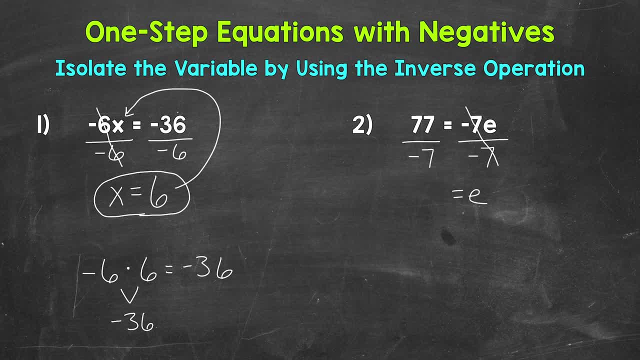 isolated, It's by itself e equals. and then on the left side of the equation we have 77 divided by negative 7. So a positive divided by a negative, That's going to equal a negative, So we get negative 11.. e equals negative 11. And we can rewrite this with the variable coming first. 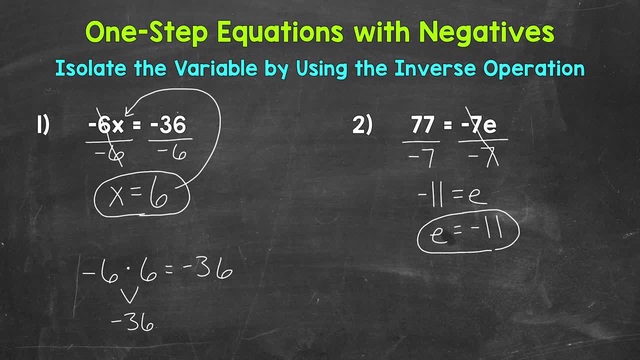 So e equals negative, 11.. Let's check that. So we have 77 equals negative, 7 times negative, 11.. We have a negative times a negative Negative 7 times negative, 11.. A negative times a negative equals a positive, So negative 7 times negative. 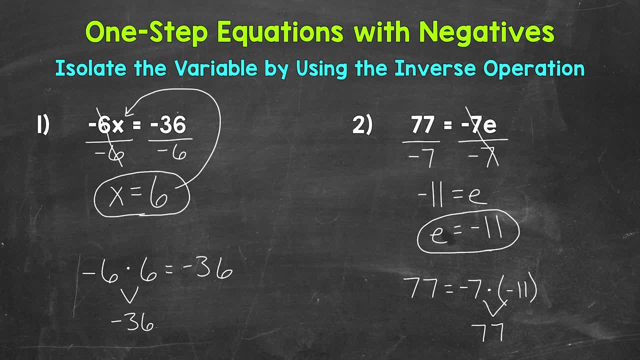 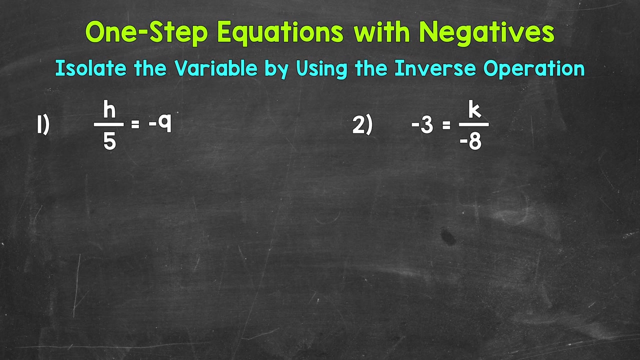 11 does equal 77.. A positive 77. We have the correct solution: e equals negative 11.. There's how we solve one-step multiplication equations with negatives. Let's move on to division. Here are our examples of one-step division equations with negatives. Let's jump into number one, where we have h divided by 5. 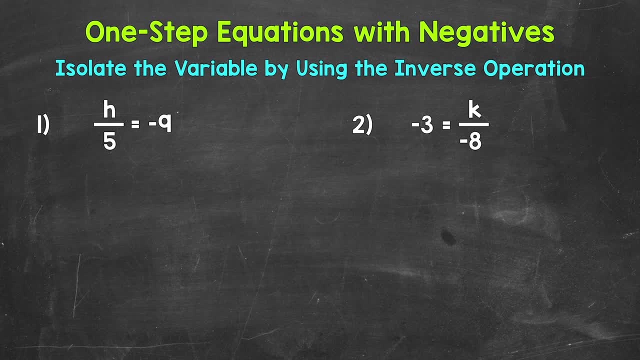 equals negative 9.. Now we need to isolate that variable. We need to figure out what h equals. Since h is being divided by 5, we need to undo that division by using the inverse operation. So the opposite operation, The opposite of division. 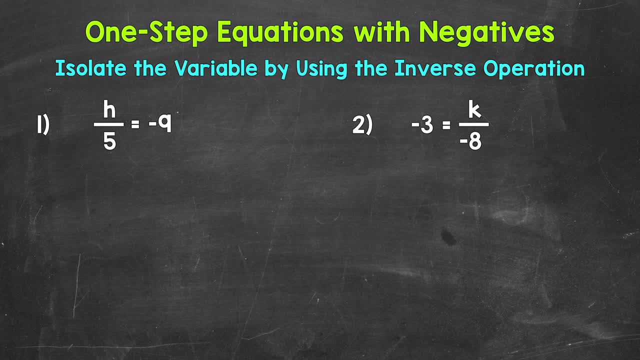 is multiplication. So let's multiply the left side of the equation by 5.. Now, whatever we do to one side of the equation, we must do to the other. In this case, the right side was divided by 5 in order to keep it balanced and equal. 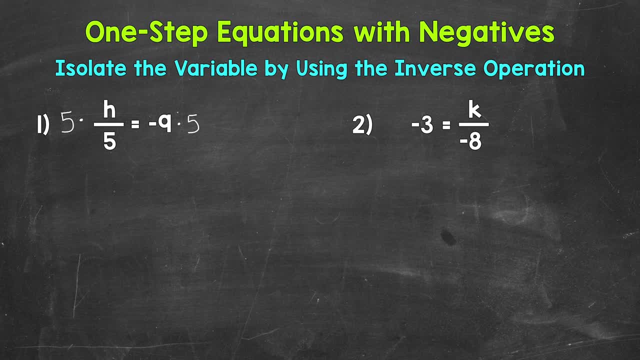 Now let's take a look at the left side of the equation. We are dividing by 5 and multiplying by 5.. So these 5s cancel out. They equal 1. Because when we multiply h divided by 5 by 5, we end up with 5h over 5.. 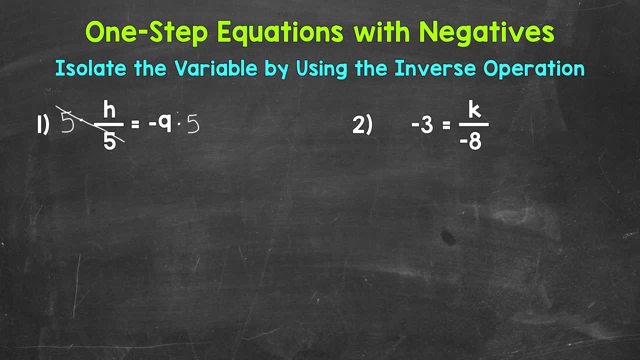 We have 5 divided by 5, which gives us that 1.. And then we have the h. We end up with 1h, which is just h. Our variable is now isolated. h is by itself, So h equals. 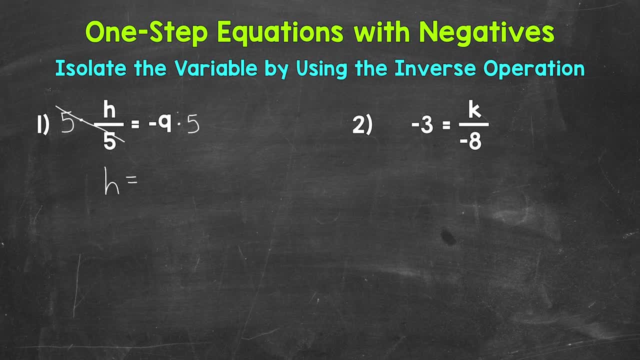 And then on the right side of the equation, we have negative 9 times 5. We have a negative times a positive, which equals a negative. So this equals negative 45. h equals negative 45. That's our solution. Now we can always check a solution by plugging it into the original equation. 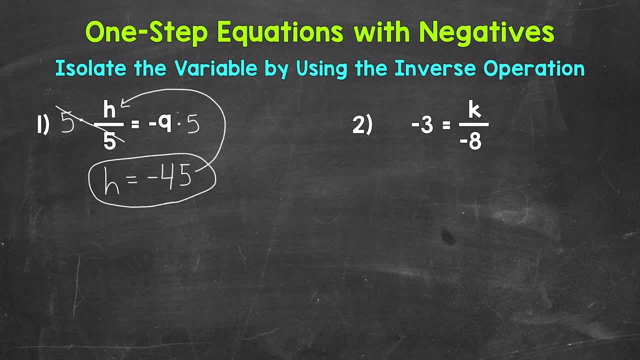 So let's plug negative 45 in for h. So we have: negative 45 divided by 5 equals negative 9. We have a negative divided by a positive, Negative 45 divided by a positive 5. A negative divided by a positive equals a negative. 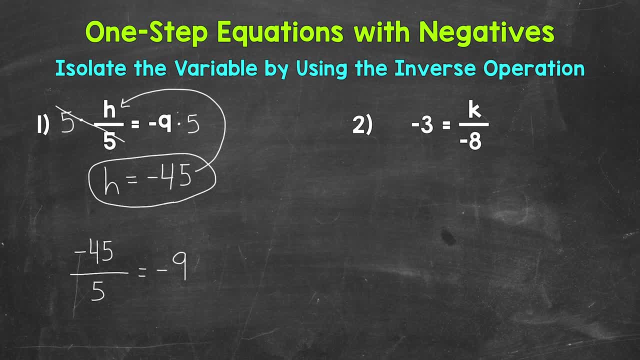 Negative 45 divided by 5 does equal negative 9.. So we have the correct solution. Now we have to multiply the left side of the equation. So we have the correct solution: h equals negative 45.. Let's move on to number two, where we have: negative 3 equals k divided by negative 8.. 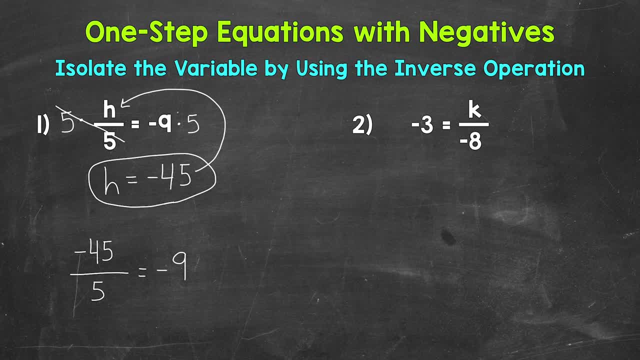 We need to isolate that variable of k. Since k is being divided by negative 8, we need to undo that division by using the inverse operation. The inverse of division is multiplication. so let's multiply the right side by negative 8.. Whatever we do to one side, we must do to the other. so let's multiply the left side by negative 8 as well. 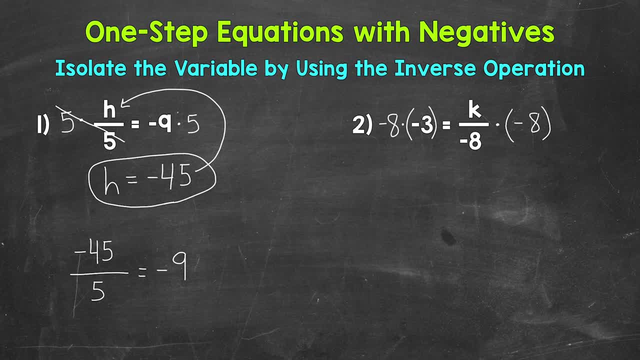 Now, as far as the right side of the equation, we are dividing by negative 8 and multiplying by negative 8.. So these negative 8s cancel each other out. They equal 1. We have negative 8 divided by negative 8.. 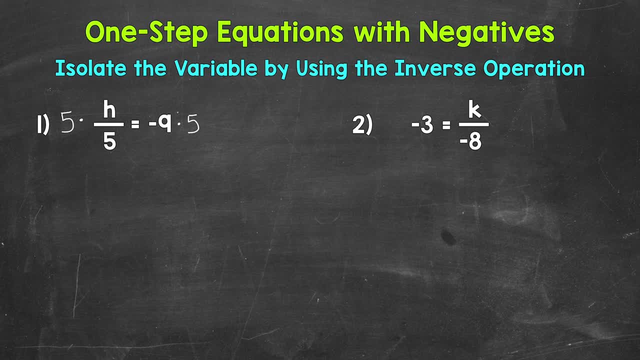 Let's multiply the right side of the equation by 5 as well. Now let's take a look at the left side of the equation. We are dividing by 5, and multiplying by 5.. So these 5's cancel out, They equal 1, because when we multiply, h divided. by 5, by five, we end up with 5h over 5.. We have 5 divided by 5.. So h divided by 5 equals 5.. We have 5 divided by 5.. So we re-calibrate. Let's add up relative equations with these. 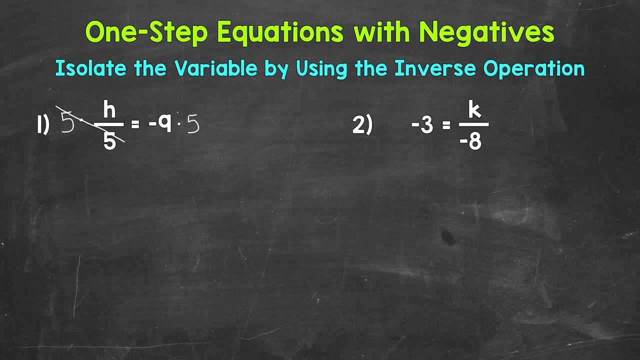 five, which gives us that one. And then we have the H. We end up with one H which is just H. Our variable is now isolated. H is by itself, So H equals. and then on the right side of the equation, we have negative nine times five. We have a negative times a positive, which equals. 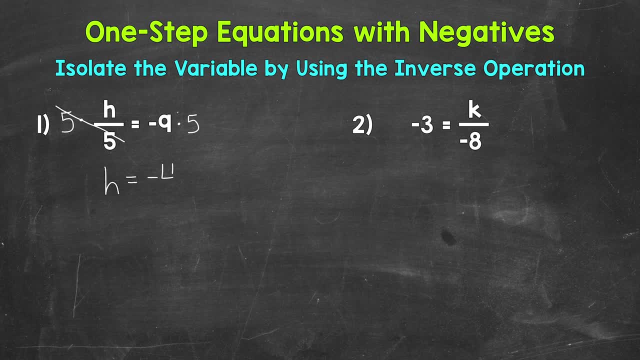 a negative. So this equals negative 45.. H equals negative 45. That's our solution. Now we can always check a solution by plugging it into the original equation. So let's plug negative 45 in for H, So we have negative 45 divided by five equals negative nine. 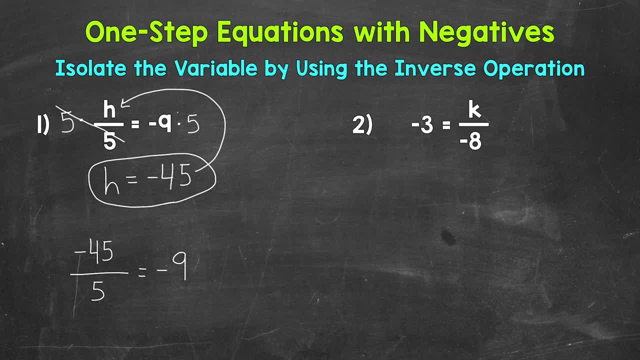 We have a negative divided by a positive Negative 45 divided by a positive five. A negative divided by a positive equals a negative Negative. 45 divided by five does equal negative nine. So we have the correct solution: H equals negative 45.. 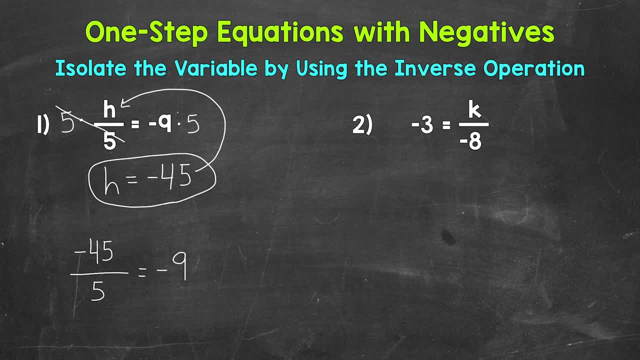 Let's move on to number two, where we have negative three equals K divided by negative eight. We need to isolate that variable. Since K is being divided by negative eight, we need to undo that division by using the inverse operation. The inverse of division is multiplication, So let's multiply the right side. 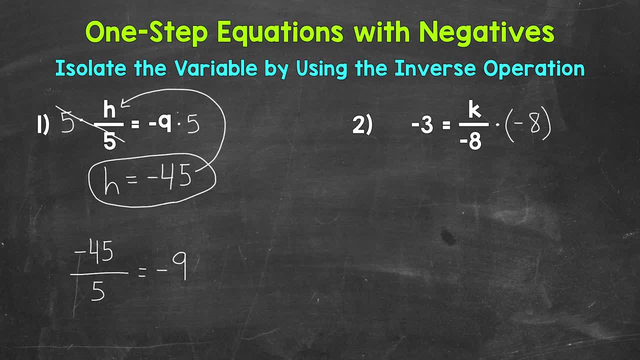 by negative eight. Whatever we do to one side, we must do to the other. So let's multiply the left side by negative eight as well. Now, as far as the right side of the equation, we are dividing by negative eight and multiplying by negative eight. So these: